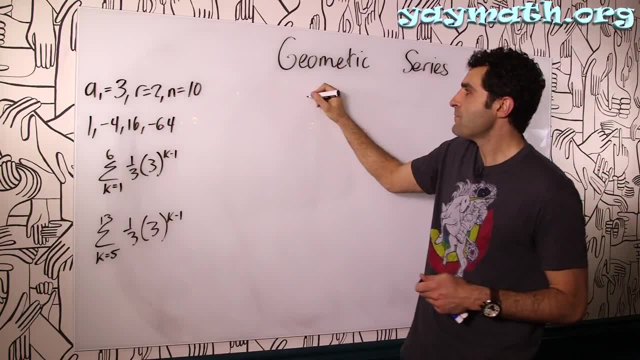 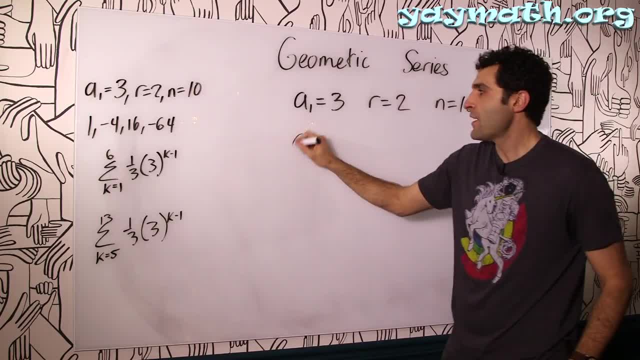 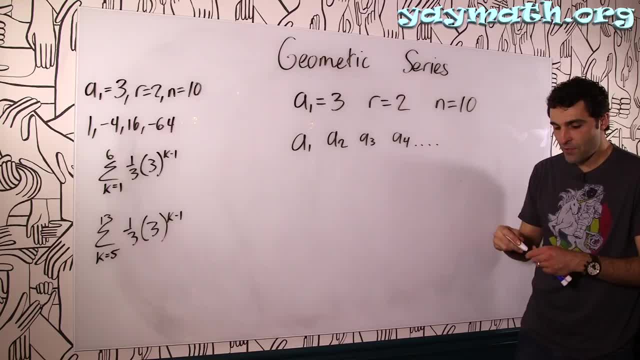 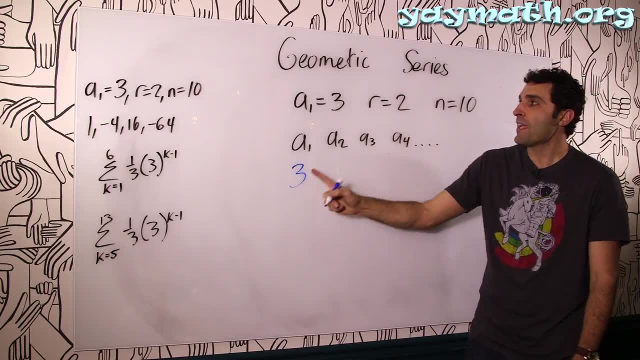 We can even write a1,, a2,, a3,, a4, and so forth. The first term in the sequence is the number 3.. We'll put that down, The ratio between them, or the rate between them of multiplication, because it's geometric. 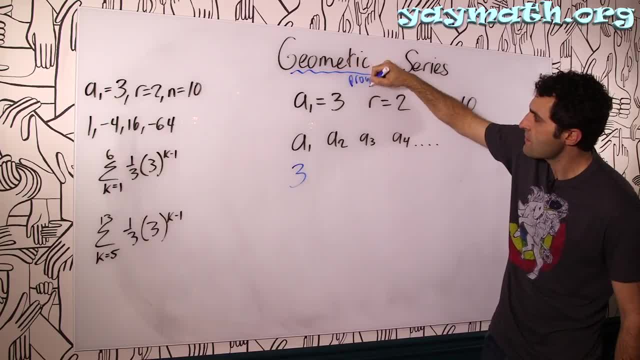 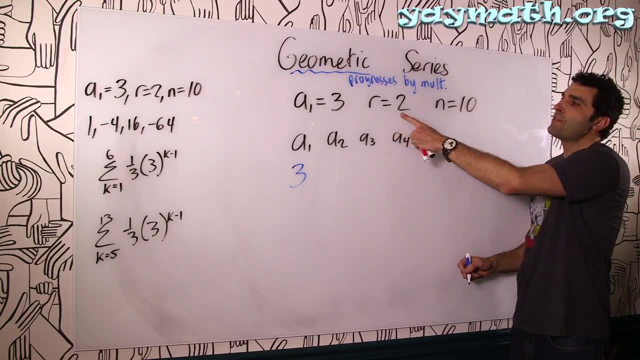 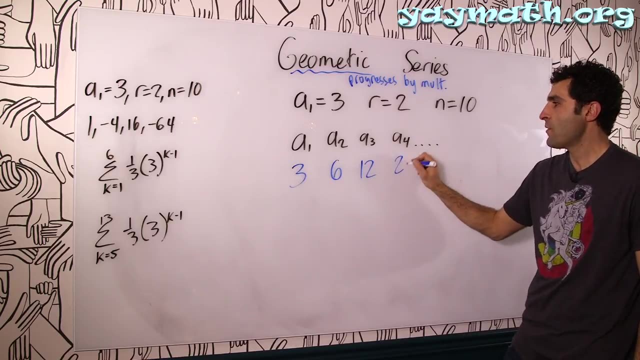 A geometric sequence progresses by multiplication. Okay, so the rate between them is times 2, so that would be 6,, that would be times 2, 12,, that would be times 2, 24.. And n is 10, meaning the number of terms is 10.. So we're going all. 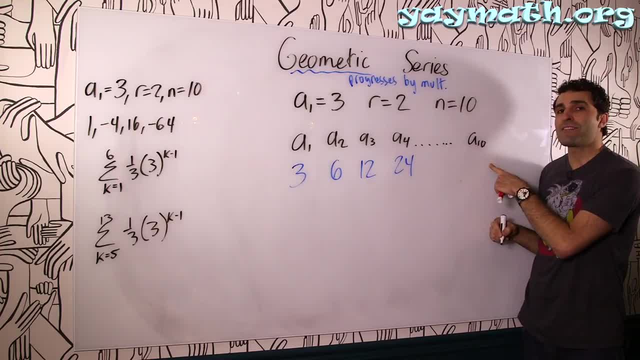 the way down here to a10, whatever that number is All right. so you can already see that would be kind of a drag. It would be a bummer to be like: all right, times 2, times 2, times 2.. 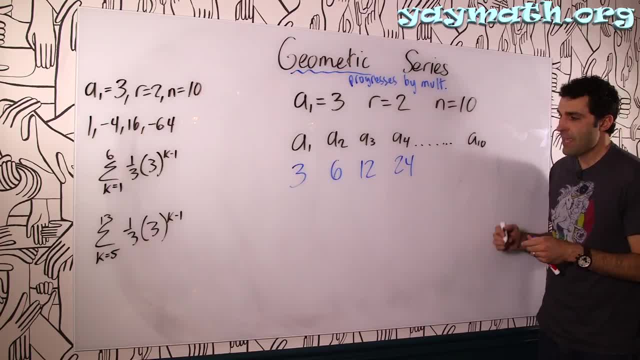 And we could do that using calculators and things like that and add them all up. It wouldn't be so bad with the calculator, because you just do times 2, maybe 6 more times and then you get this number here. okay, This is a geometric sequence. A geometric series means add all terms. Why do I? 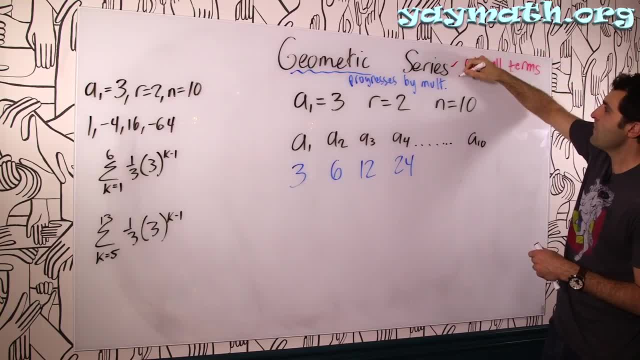 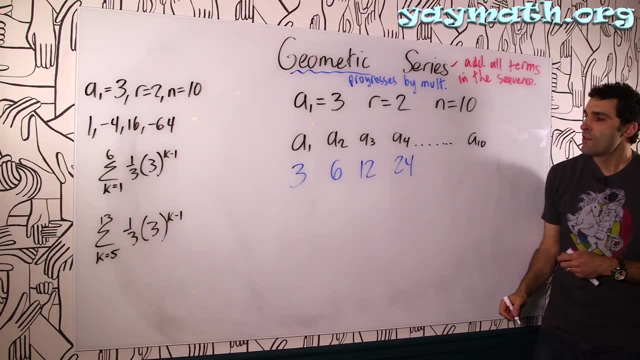 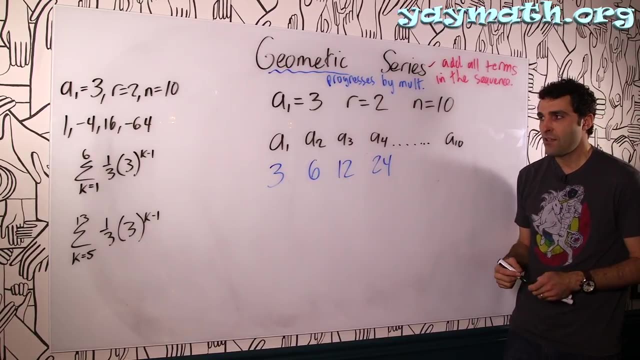 say it like this: Well, I can't stop now. Add all terms in the sequence. There you go. Add all terms in the sequence. So we could do this manually. It would be a bummer. I don't want to do it. I'm going to offer you a formula now for a geometric series. It's the. 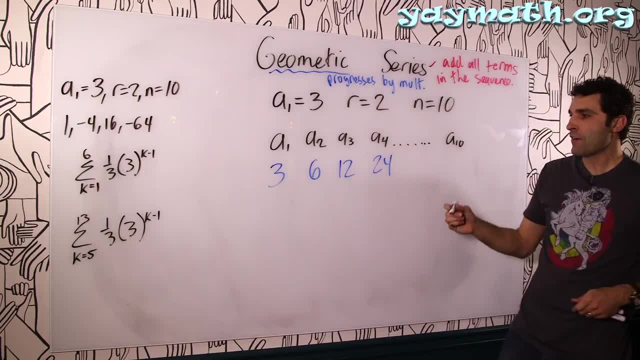 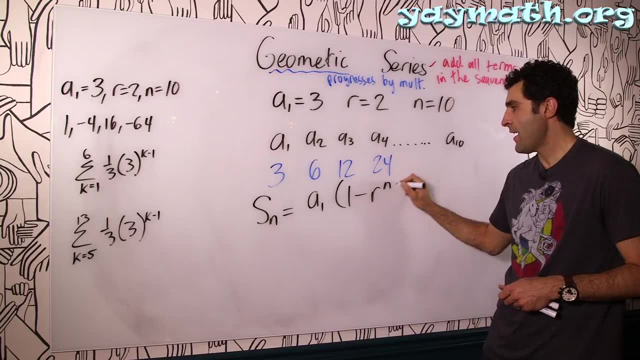 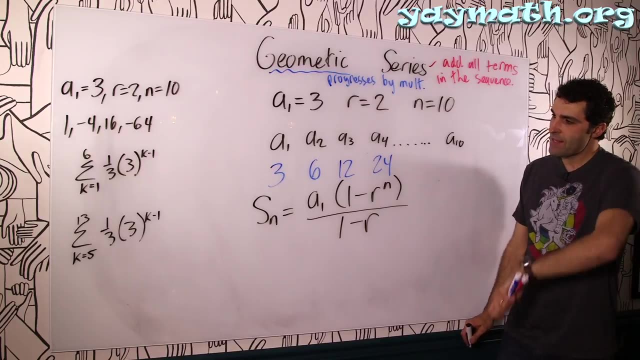 sum of geometric sequence. adding all these up, Here's how it goes: Sn is a1 times 1 minus r to the n all over 1 minus r. All right, so this is the formula that's offered in the books. Let's analyze This: is the sum of the first n terms that we seek. In this case, n is 10,. 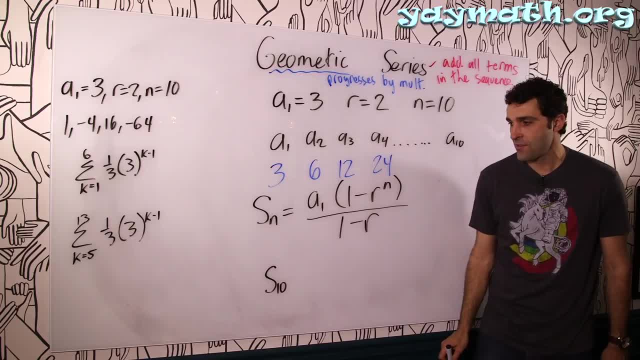 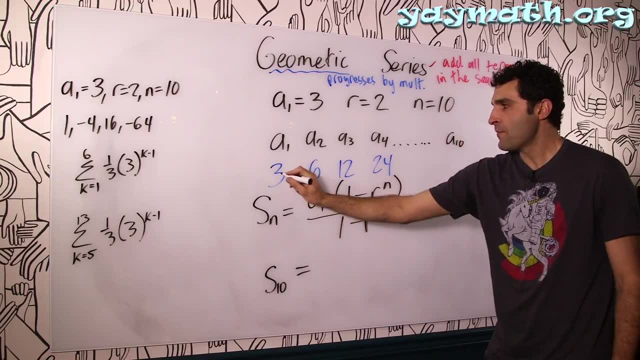 so this would be s10, the sum of the first 10 terms. Students tell me that my s's look like fives. Apologies in advance. Here we go. a1 is the first term, 3.. 1 minus the rate of change, 2.. 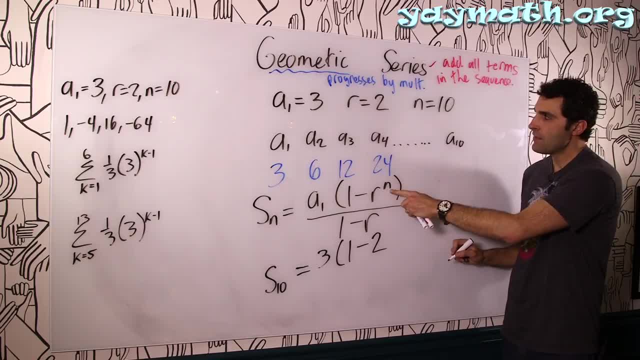 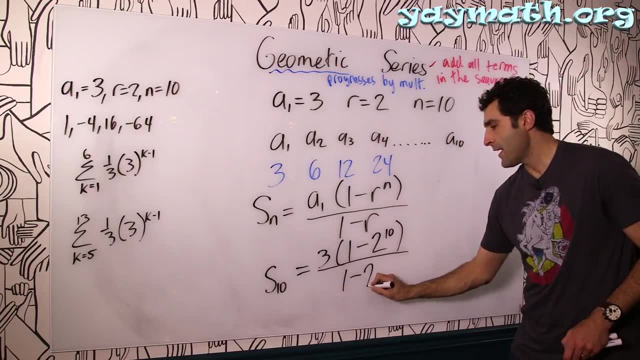 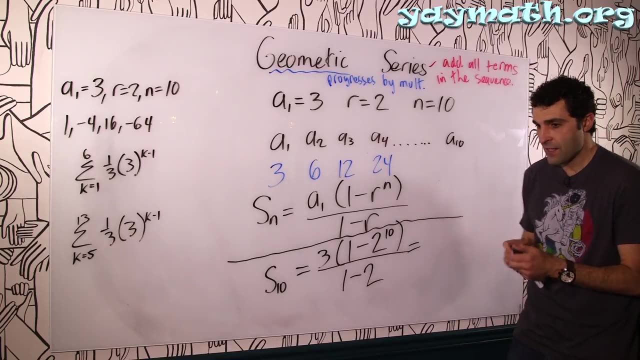 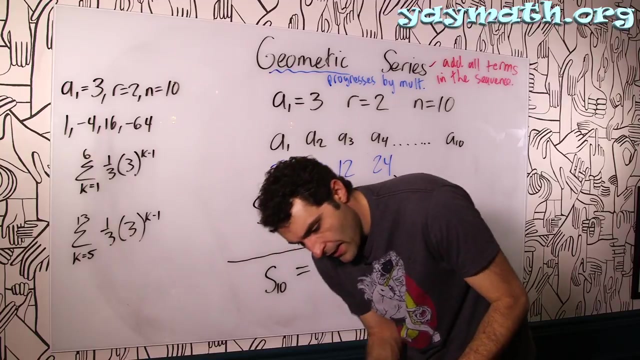 2 to the n. Oh, n is 10. again, All over, 1 minus 2. again. Pay a little space. There you go, All right. So yeah, we do need calculator for this. I think I brought mine over here. All good, Okay, All right, get. 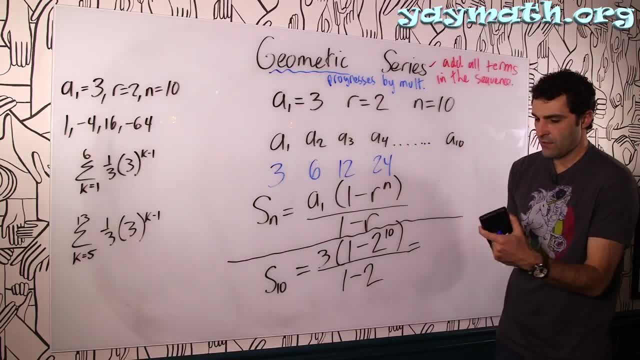 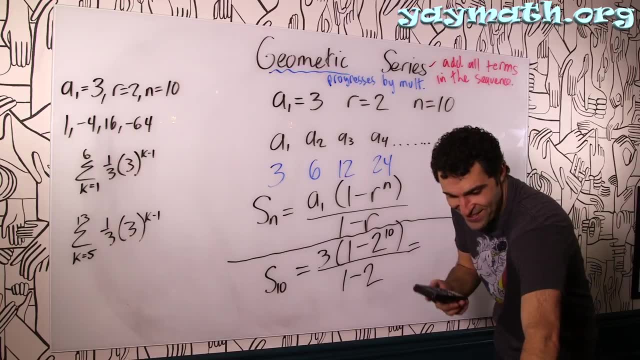 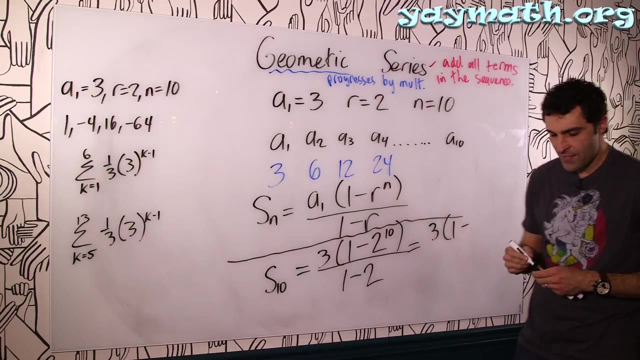 a calculator, All right. So let's put this in: Your batteries are low. Recommend change of batteries. Thank you, Texas Instruments. That is actually cool. They put that in. All right, so this is 3.. 1 minus 2 to the 10.. Put it in On 2 to the. 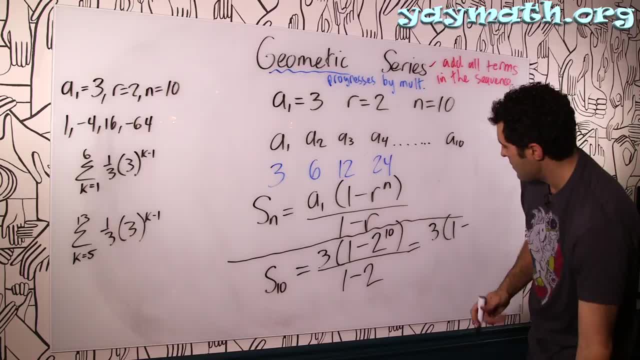 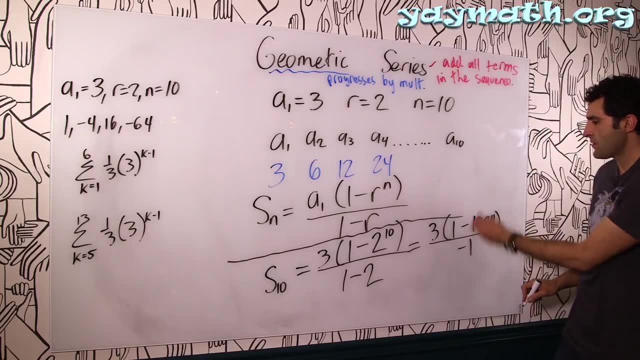 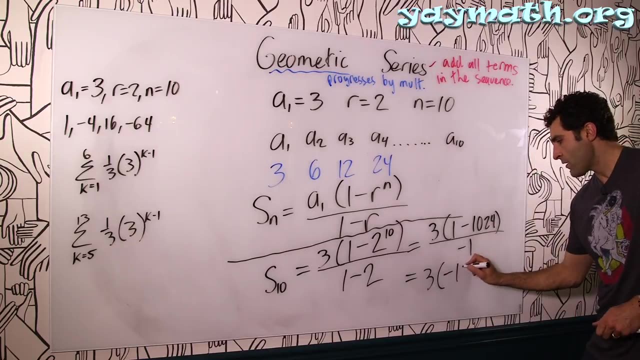 10. 1024.. 1 minus 1024.. All over 1 minus 2 is negative 1, so ultimately we're going to divide by negative 1.. This is 3 times 1 minus 1024 is negative 1, 0, 2, 3.. 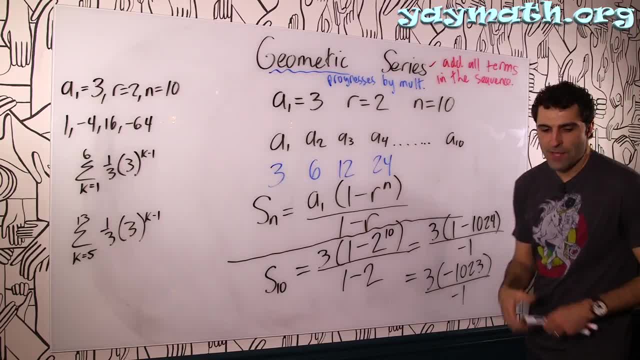 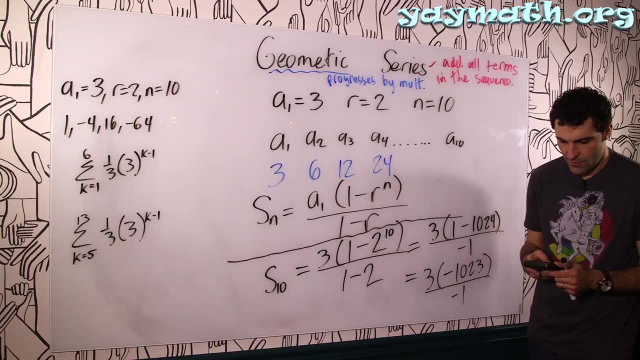 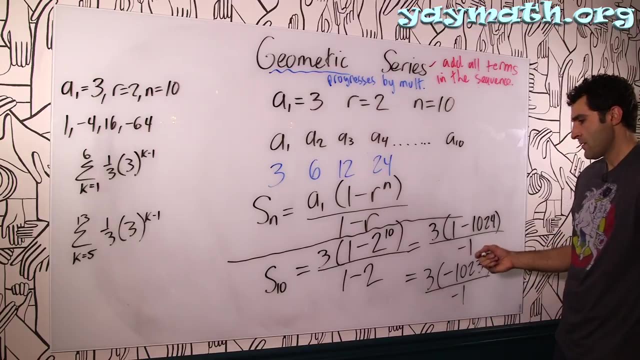 All over negative 1.. All right, multiply those 3 times 1023.. 3 times 1023.. 3069.. So you'll notice the top will be negative. Divided by negative 1 is 30.. 3069.. I'm telling you a true. 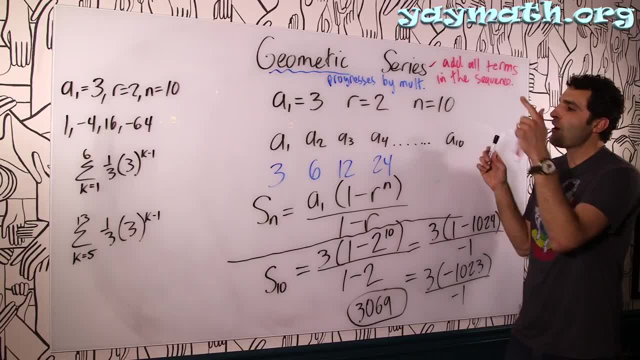 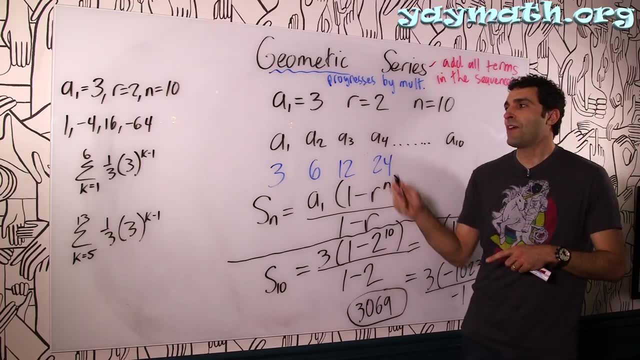 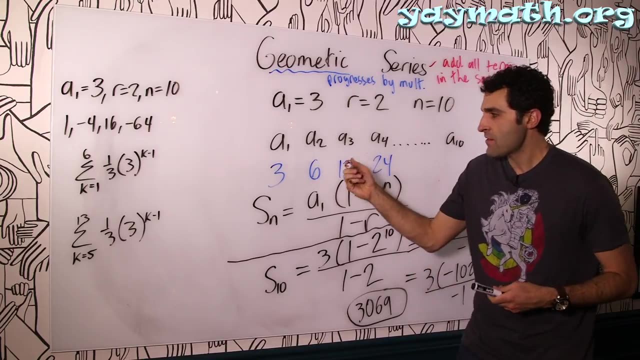 story Dollars to donuts- 100% true. I would offer a problem like this on a test or even an exam And there would be students- bless them- that recognized what a geometric series was. Is that basically adding a bunch of terms in a sequence, So this person, or multiple? 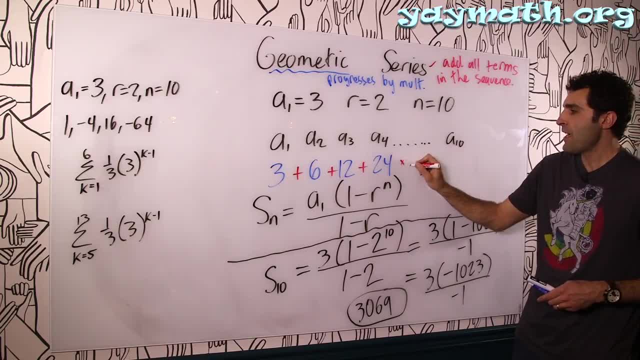 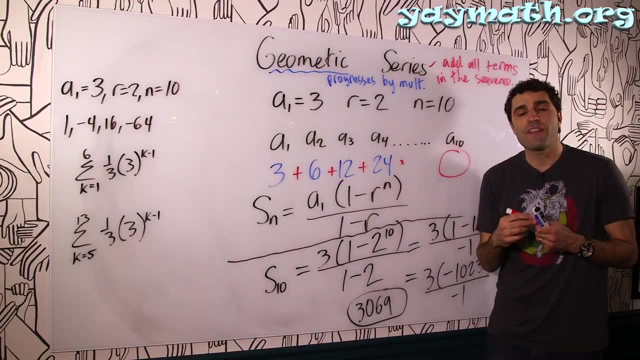 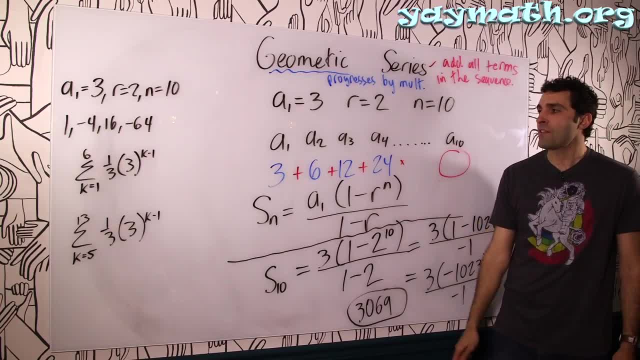 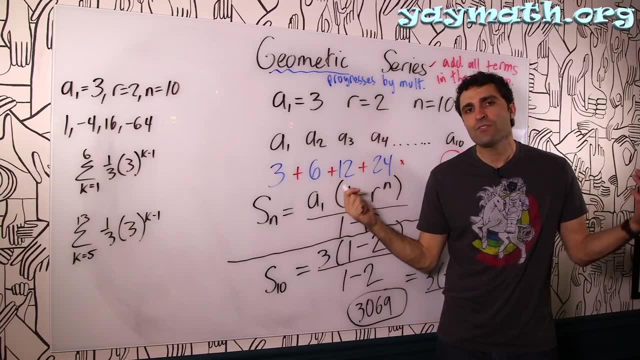 know sort of bogged down by only using the formula. If you understand the process of adding a geometric sequence, adding up all the terms, then you could sidestep the whole need for a formula. But what if I asked for n equals 100 or n equals 500 or something? 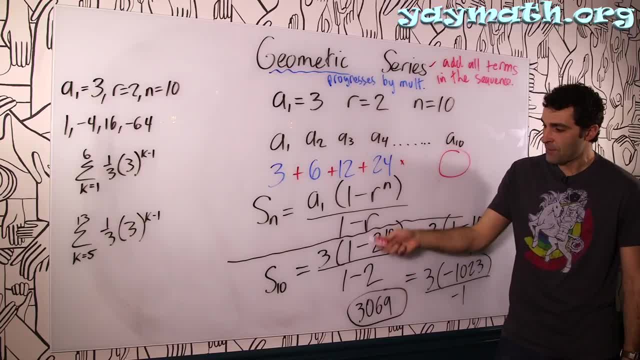 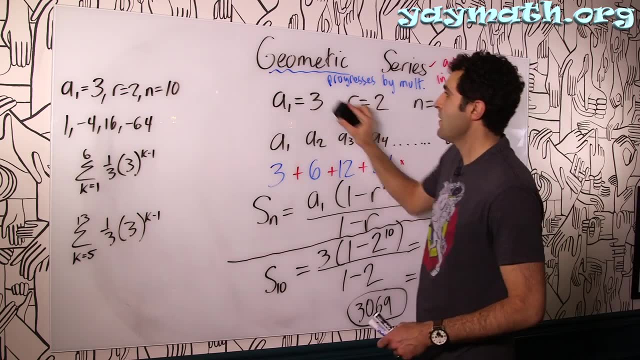 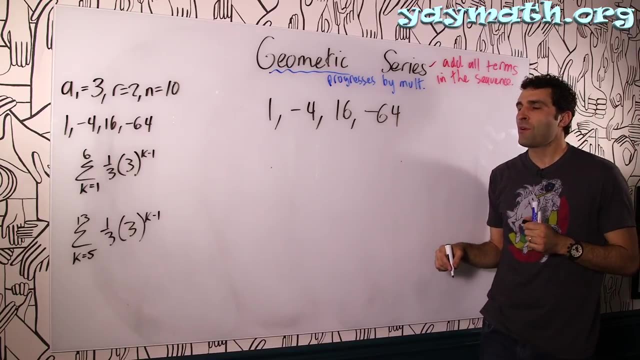 like that. It would be really helpful to have that calculator and being able to use the formula to do it Right. But I just wanted to point that out. That's kind of cool. they did it that way, Okay. So in that spirit, I actually want to do this problem both ways. I want to do it with the. 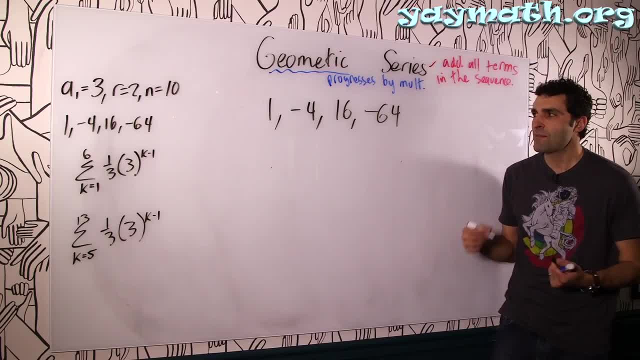 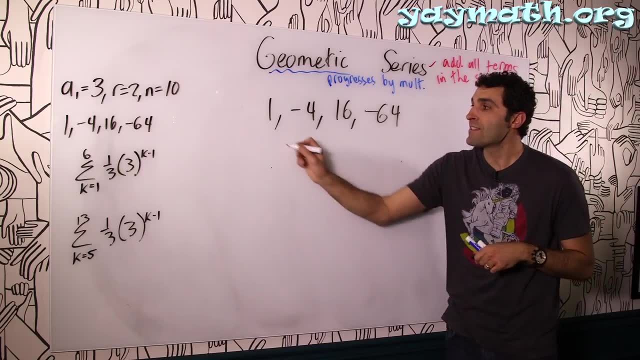 formula and I want to do it manually and see if we get the same thing Right. There's something very satisfying about that- to make sure that everything aligns. So let's get the sum of this geometric sequence. We can see that this is geometric because it does progress by multiplication. 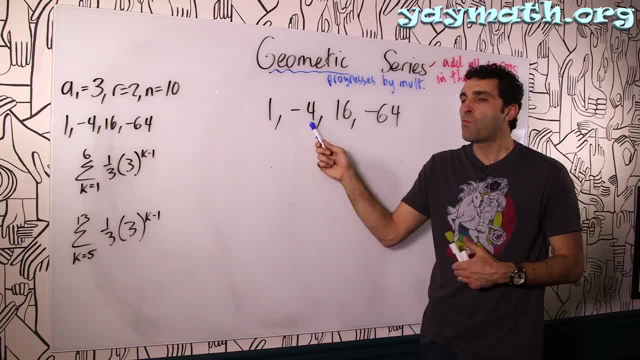 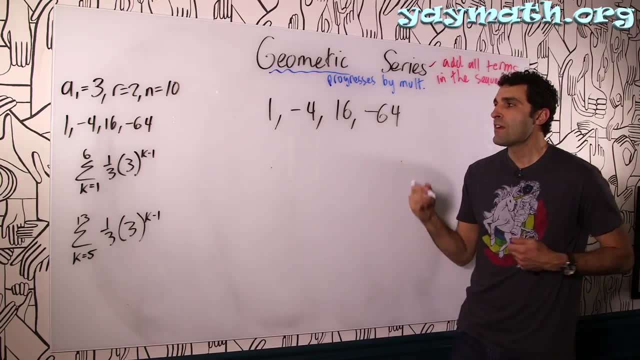 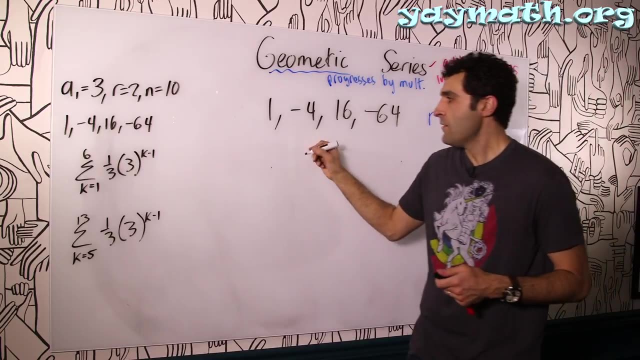 What are we multiplying by each time? Look closely: 1 times what is negative: 4? Negative 4 times what is positive: 16?. 16 times what is negative: 64? 16.. R is negative 4.. Right, So let's go ahead and do it with the formula: S4 equals. let's. 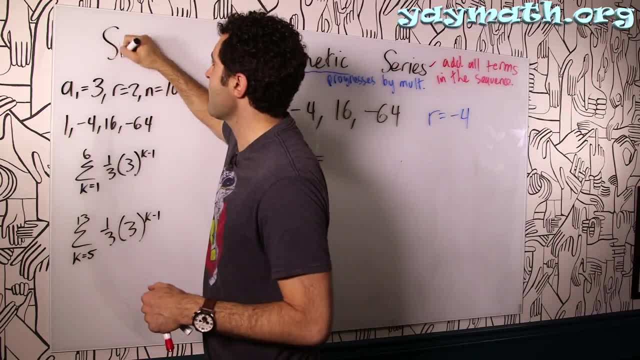 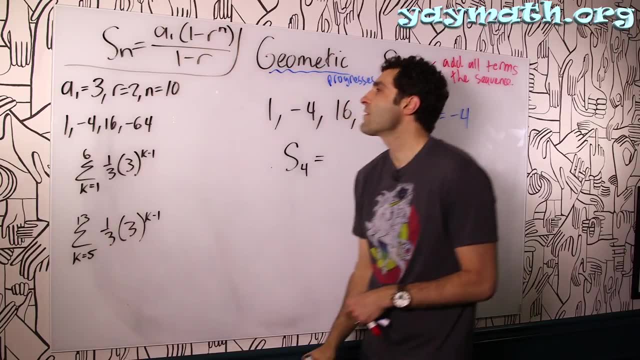 go ahead and jump right into the actual action. I'll put it over here: Sn equals a1, 1 minus r to the n all over 1 minus r. So we have that as a reference. Now we can use it over. 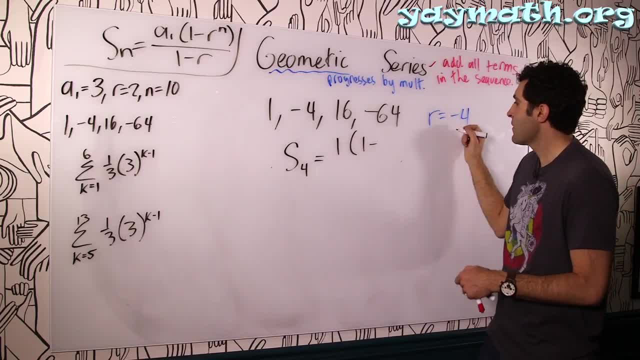 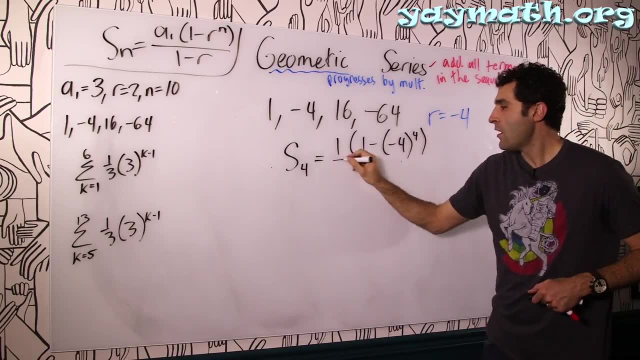 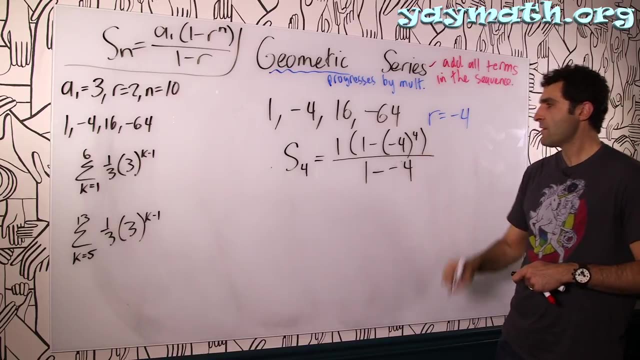 there. First term: 1, 1 minus negative 4.. This is cool. I'm glad this is happening To the 4.. Sure, All over, I get that. Yeah, All over: 1 minus negative 4.. Okay, So we have to follow order of operations here. It's tempting to say that. 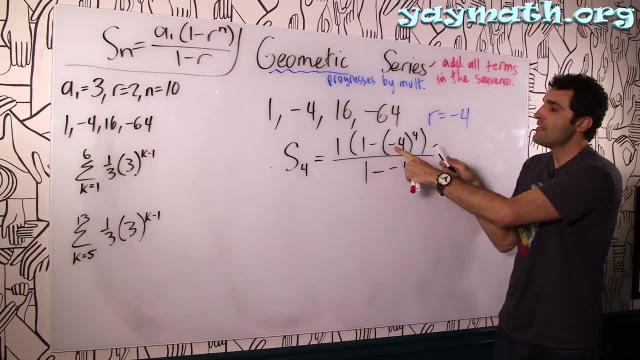 these two cancel but they do not Right. The negative 4 is bounded by this exponent, So the negative 4 to the 4th will be positive, but we'll get 1 minus that Right. The 1 is negligible. 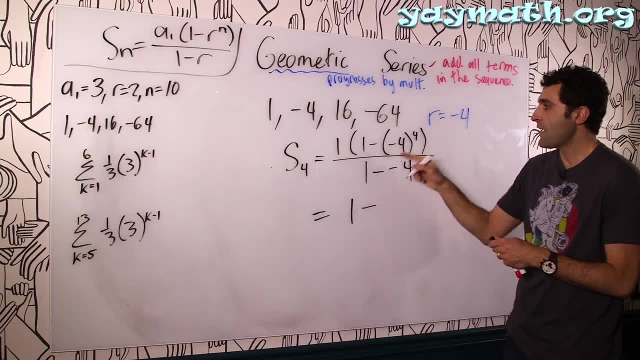 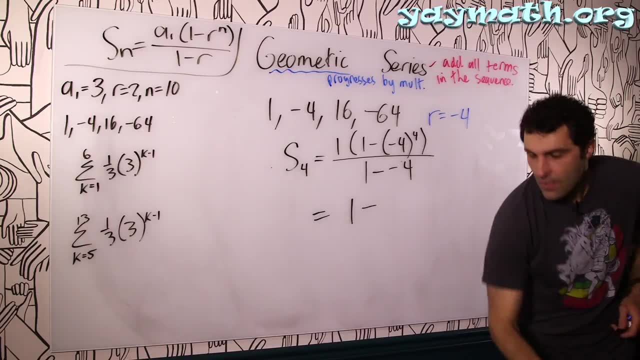 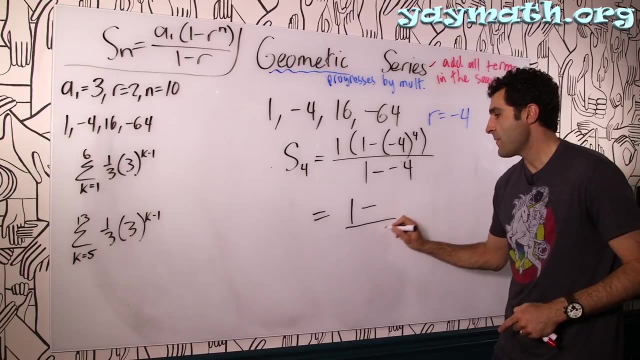 That 1's gone. This is 1 minus whatever negative 4 to the 4 is. I need that here And this does cancel 1 minus negative 4, because there's no exponent that's happening with this negative 4.. So this is going to be all over the number 5.. Let's find out what negative 4 to the 4. 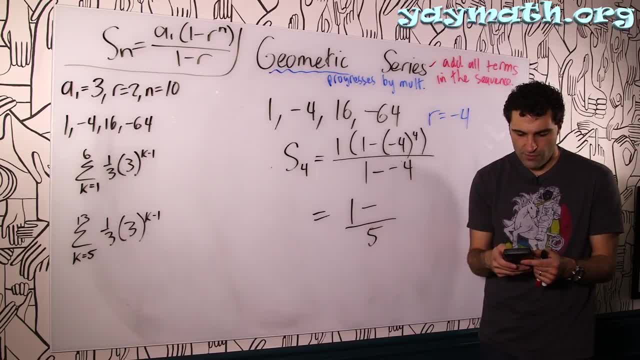 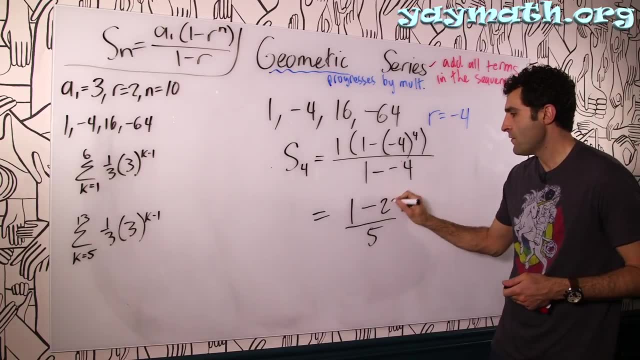 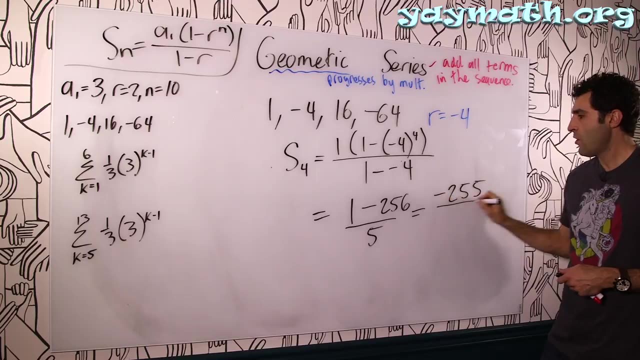 is. It's the same as positive 4 to the 4., 4 to the 4.: 256.. 256.. This is 1 minus 256, which is the same as 1 minus 256 is negative, 255 over 5.. All right. 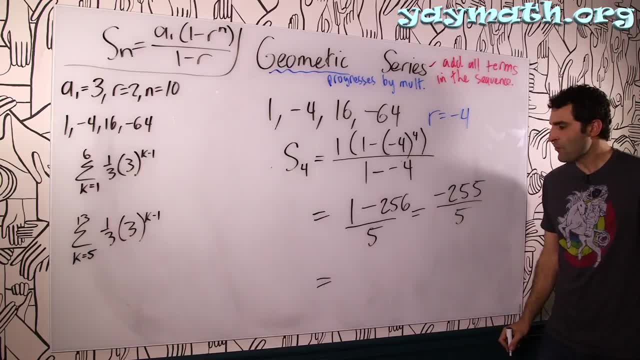 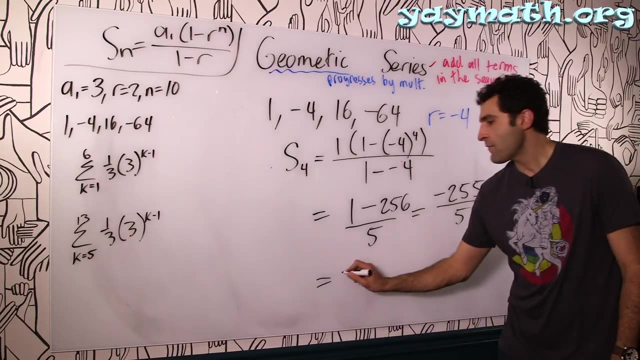 Captain, let's see if I can do this in my noodle. in my brains, 5 into 200 is 40.. 5 into 55 is 11.. So 40 plus 11 is 51, negative 51.. 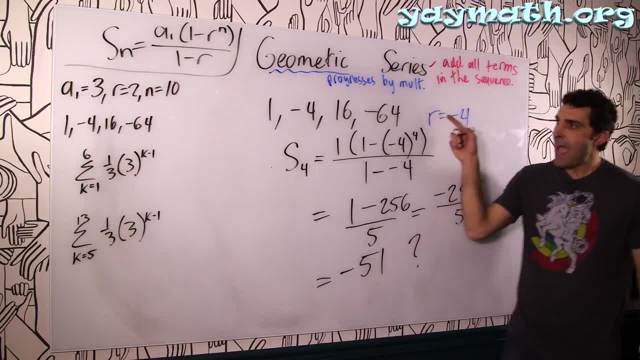 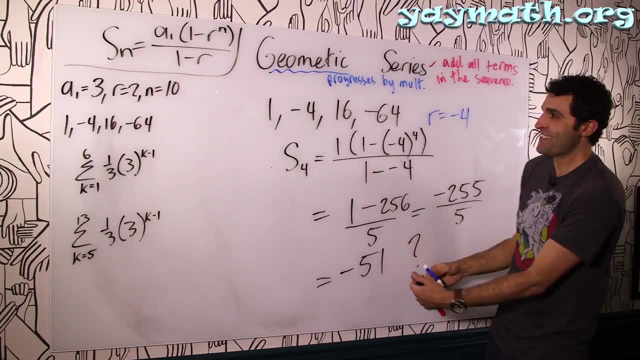 All right, Jury's out. Let's see if I did it right. Add them up. Here we go. I am physically excited. 1, I just want to see if they're the same 1 plus the. I'll actually do a better way. 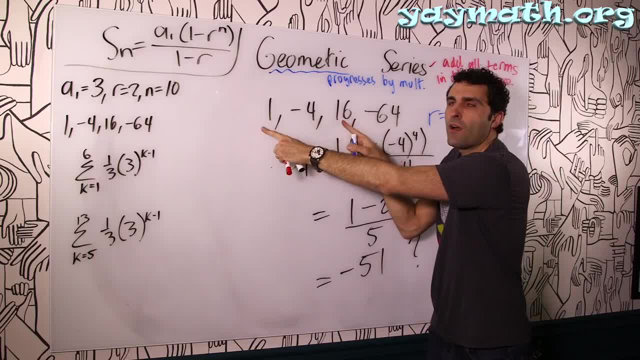 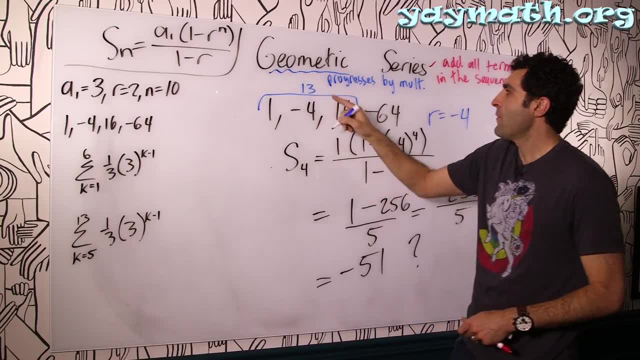 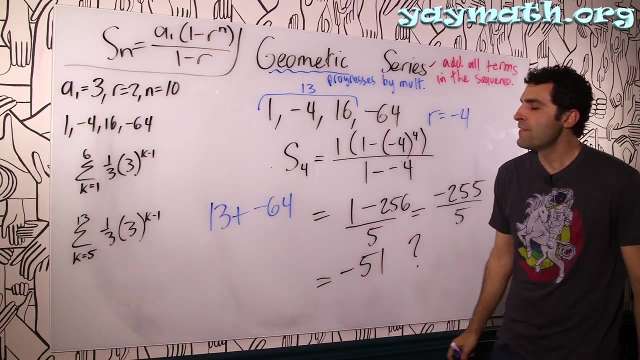 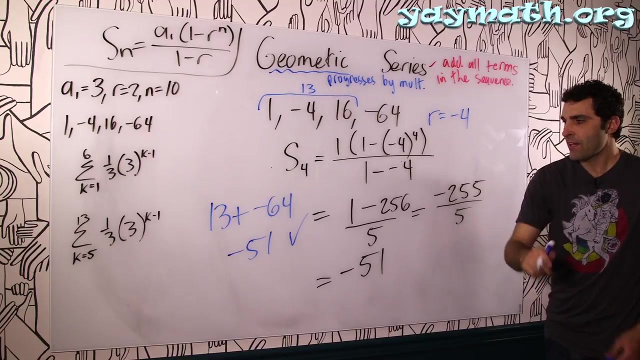 to add This would be: 12 plus 1 is 13.. Yeah, so this is 13 up here, And we've got 13 plus negative 64. And that's 50.. Yeah, negative 51.. All right Score. Yes, All right. Cool, So it worked both. 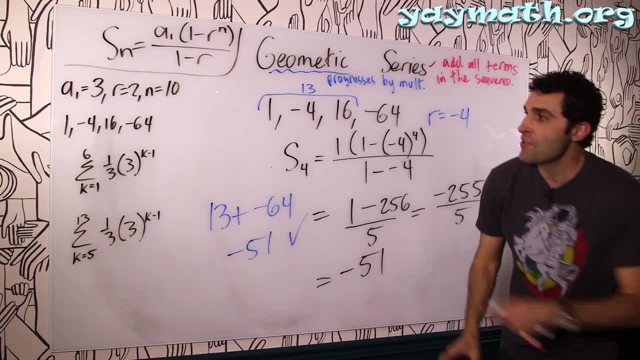 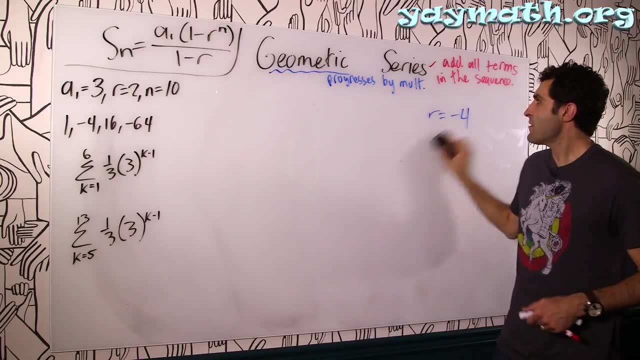 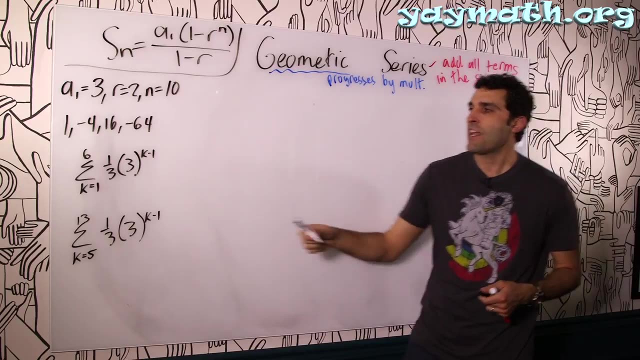 ways, Something very satisfying about that. All right, Let's introduce you to sigma notation here. One of the reasons- right, I'll just introduce it while I'm even erasing One of the reasons I've enjoyed doing in-studio with you is that I get a chance to introduce this. 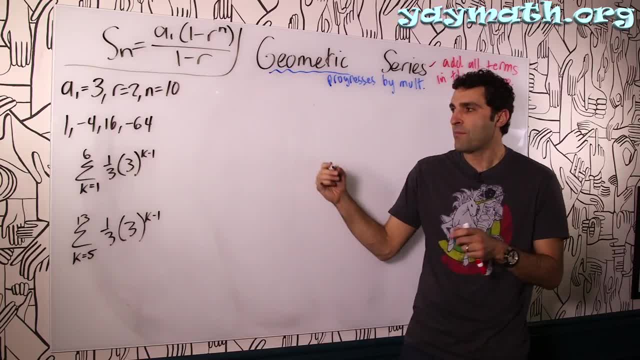 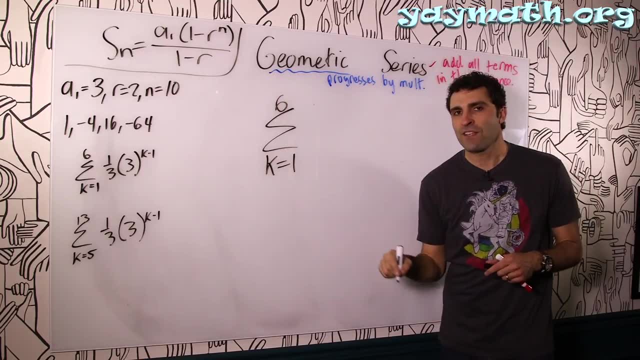 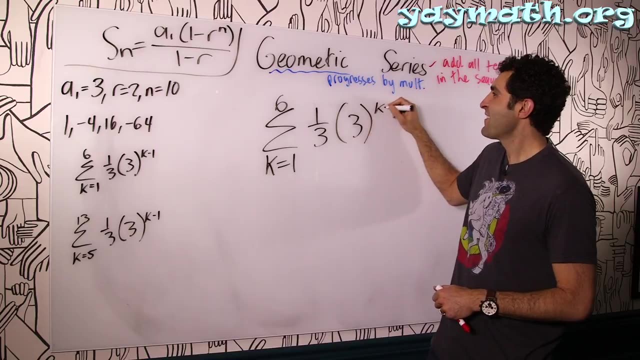 high-level stuff right In a way that makes sense, right from the jump Anytime. you see literally Greek. it is an opportunity to run for the hills, okay, And pick olives, But we're not going to do that, all right. 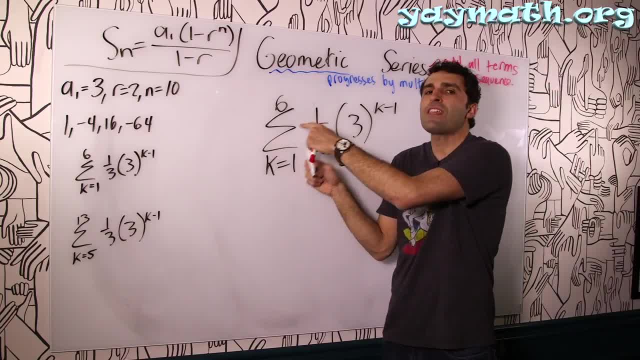 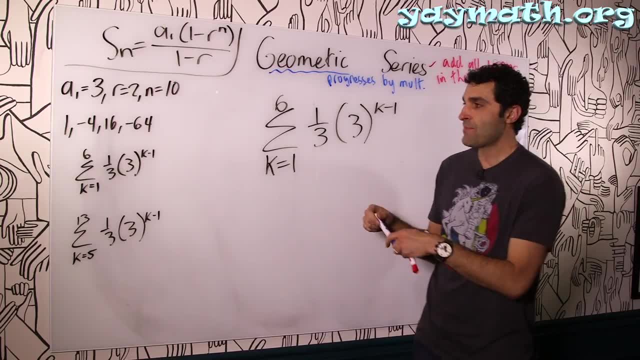 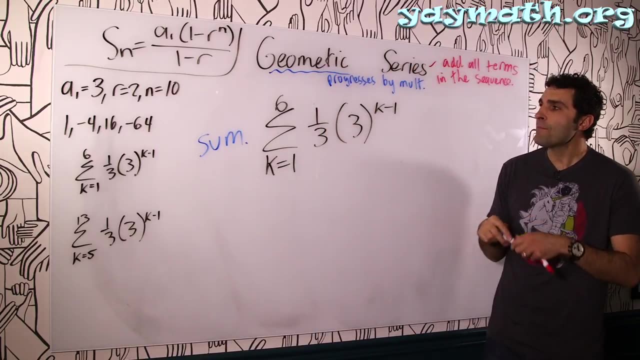 Because we're going to explain what this means. This is the Greek symbol, sigma, It's capital sigma. Sigma in math land means sum. That's it. Let's put it down: Sum Dot, That's what it means. It means the sum of every term ranging from the first term. 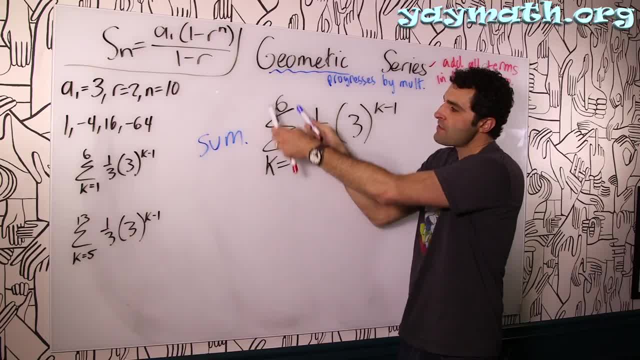 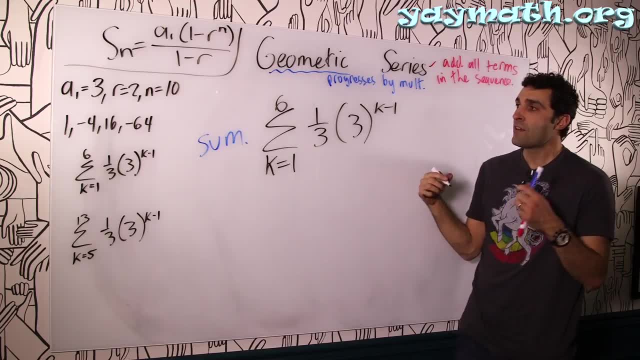 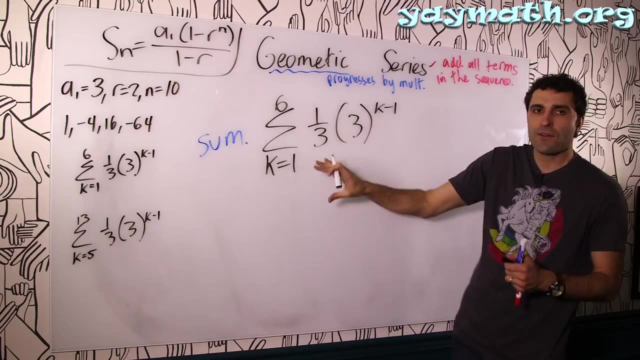 to the sixth term. So you could see in this sequence that there will be six terms, ranging from when k is 1 to k is 6.. Let's actually a really good practice. for anyone learning this stuff is to get a fix of what the sequence looks like. to actually list out these six terms: 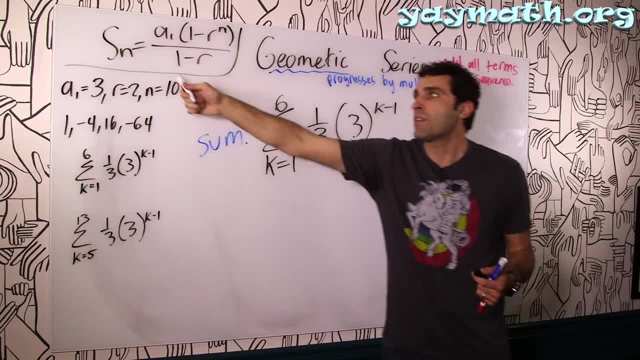 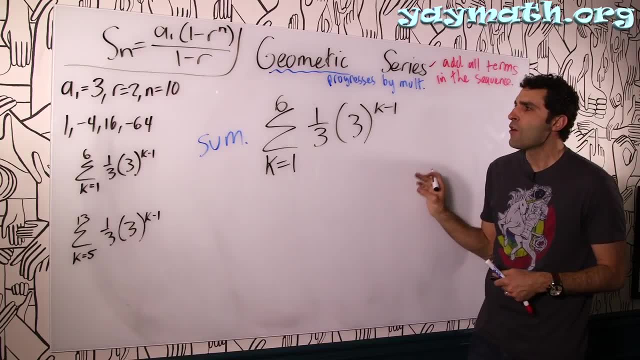 And then, if you wanted to, you could just add them up and you don't even need the formula, Or we can use the formula. Either way, I would recommend especially learning. just write out the six terms, Or at least some of them, At least the first three. 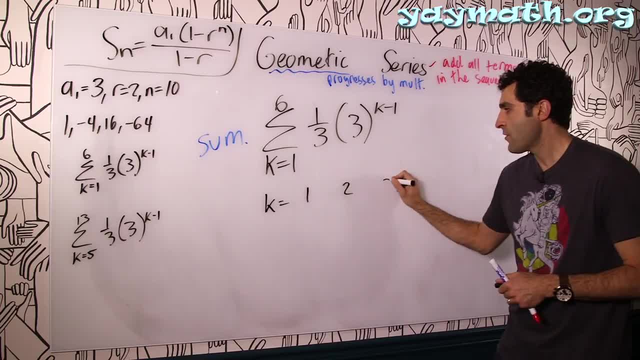 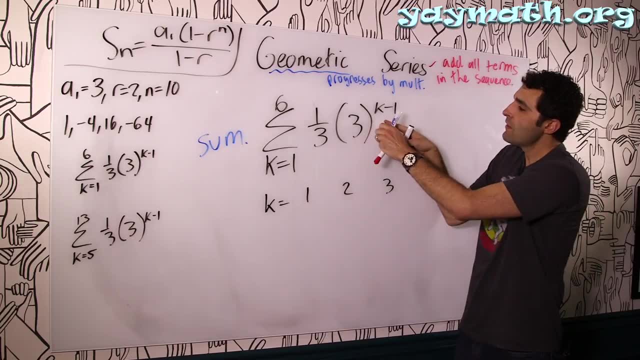 The first term in the sequence. here we go. This is k equals 1,, 2,, 3, 4.. Let's see what happens. The first term in the sequence is when k is 1.. So we go. k is 1 here. If k is. 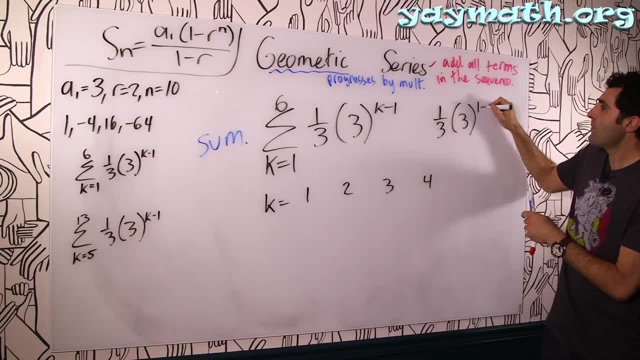 1, this would be 1 third times 3 to the 1 minus 1.. 1 minus 1 is 1 minus 1 is 0. So this is 0.. And 3 to the 0 is the number 1.. So this becomes 1 third times 1.. This is. 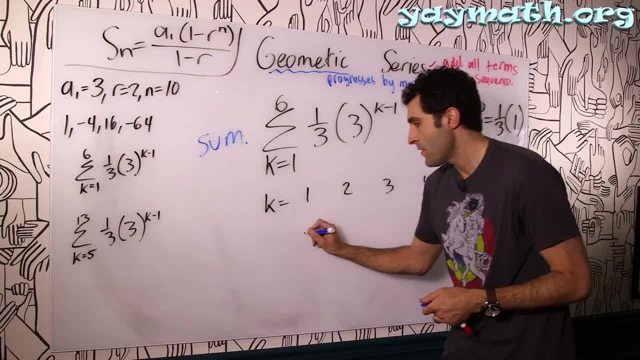 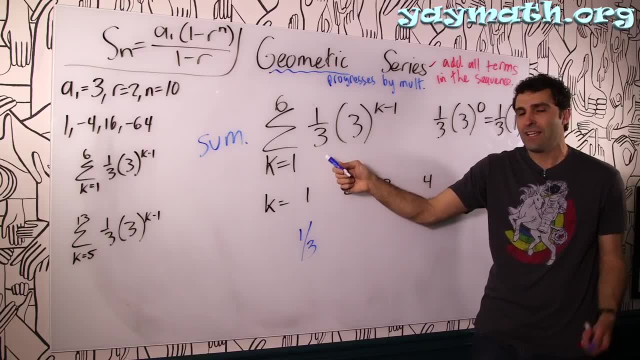 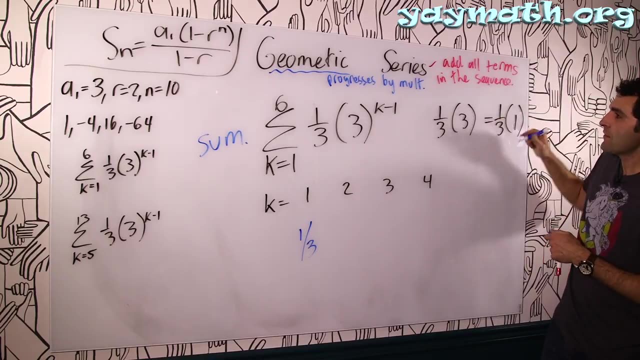 1- third. So the first term in the sequence is 1- third. Here's a big hint. Oftentimes this coefficient here is the first term. That's usually. that's a big hint, It's a giveaway. Okay, The next term in the sequence is when k is 2.. Let's put in 2 there. 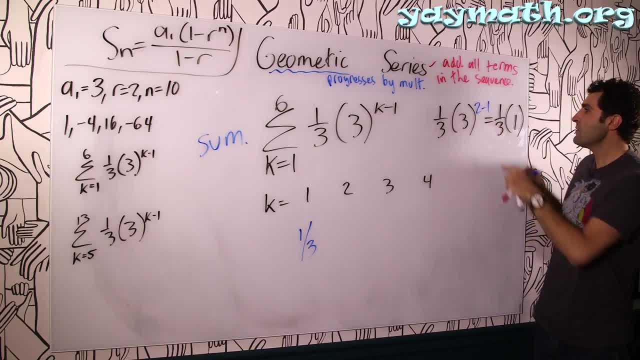 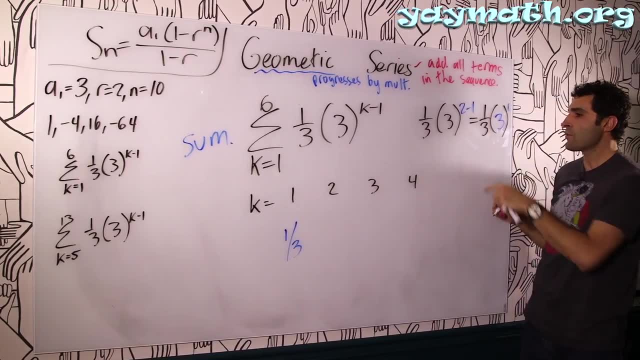 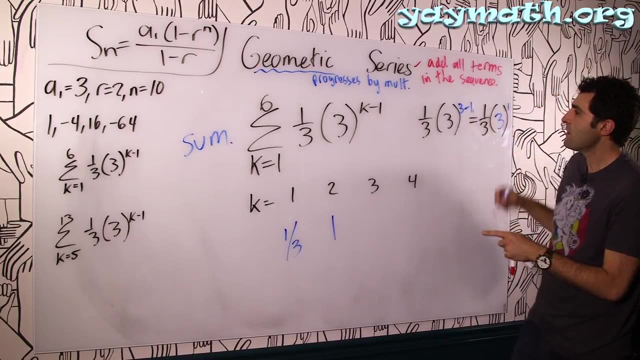 So this is 2 minus 1.. 2 minus 1 is 1.. So that becomes 3 to the 1.. 1 third times 3 is the number 1.. It goes there. Let's do it again When k is 3.. So we put 3 minus 1 here, That. 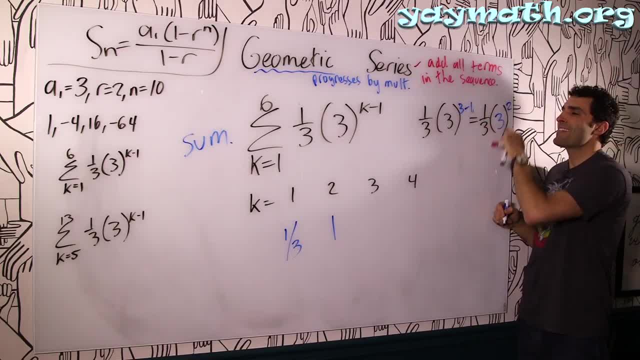 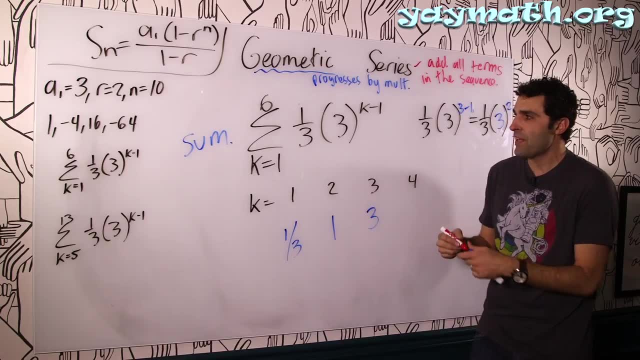 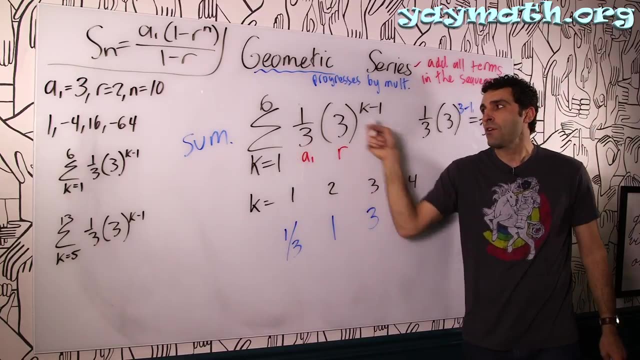 becomes 3 to the positive 2.. 1 third times 9.. 1 third times 9 is 3.. And you can see what's progressing here. This, if you look closely, embedded within This is a1.. And this is r. That's going to happen over, and over and over again. Okay. 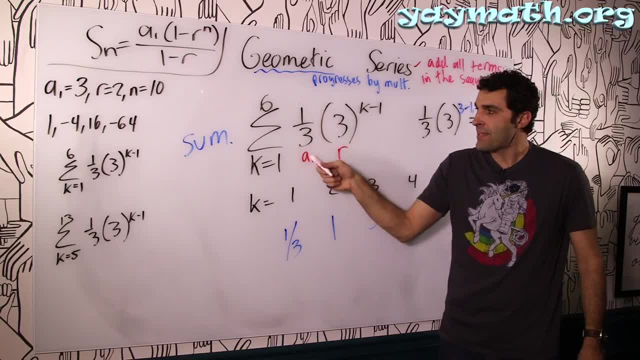 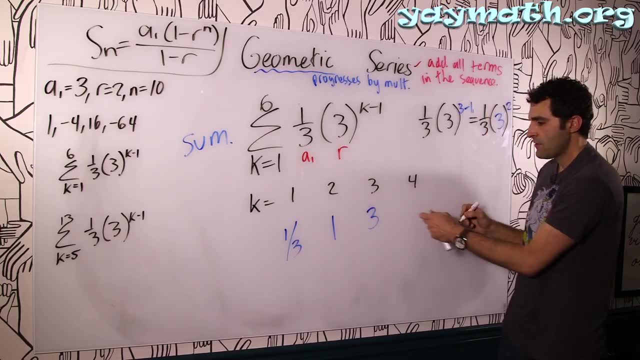 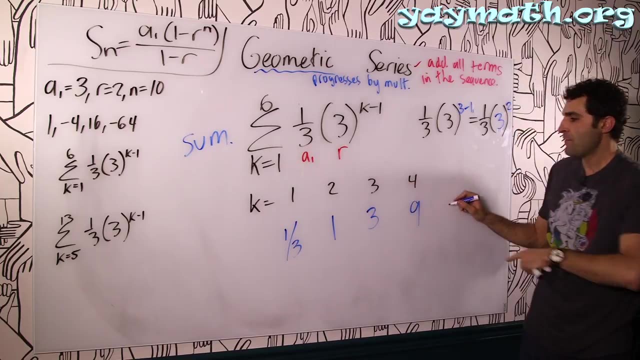 So look for those within your sequences that this is the first term and this is the rate of change, So you could even just go ahead and fast forward. Times 3 times 3 times 3 is 9.. While we're at it, let's go ahead and do times 3 again to get the fifth term is 27 times 3 again. 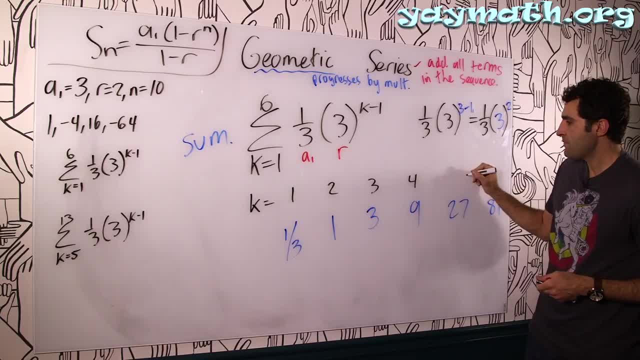 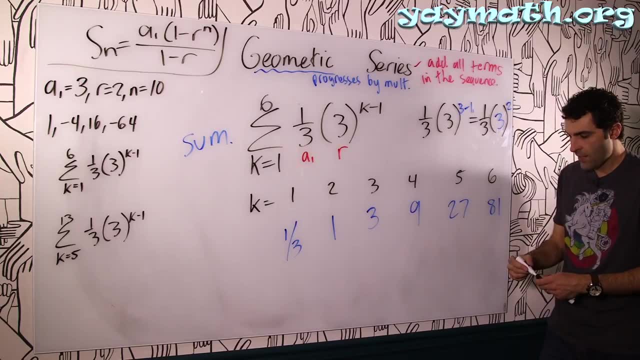 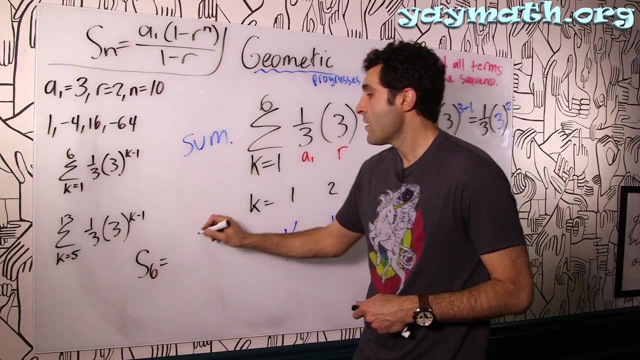 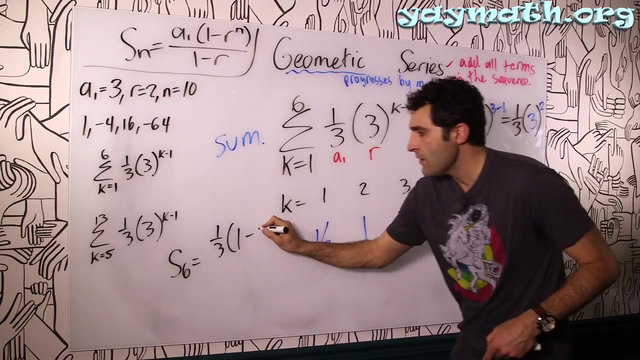 81. This is 5.. This is 6.. Sum all of these blue terms right here and the problem is done. Okay, Let's set it up using the formula. So we got: s6 equals a1, is 1. third, 1 minus the rate of change is 3 to the. 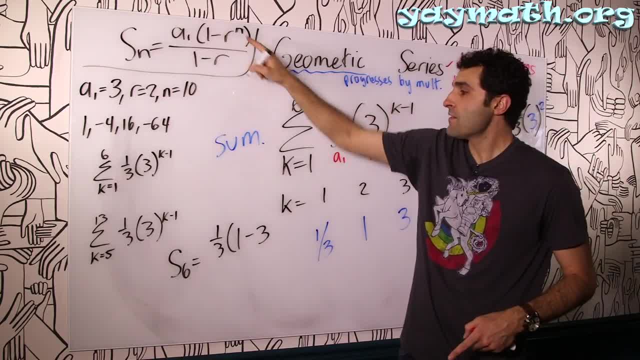 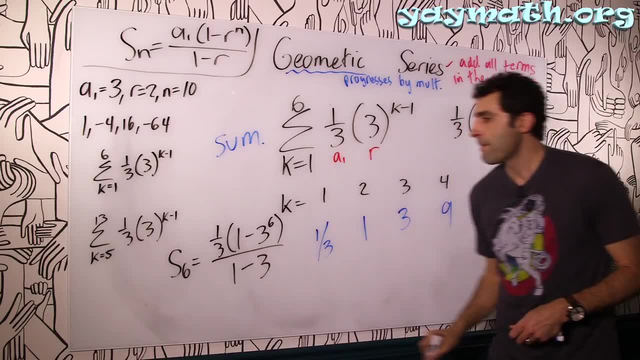 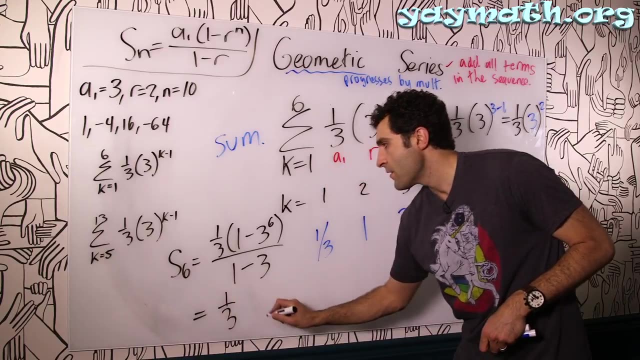 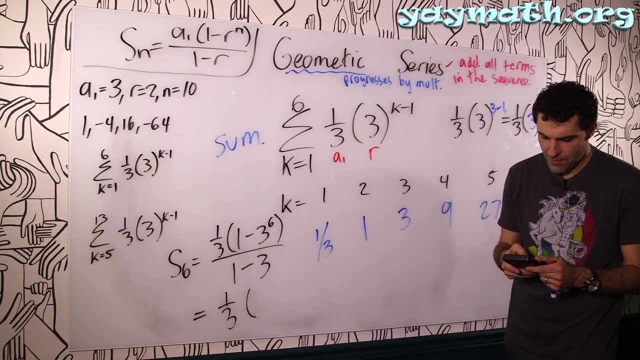 how many terms are we doing? 6.. There it is All over. 1 minus r again is 3.. Okay, Let's see what floats. This becomes 1 third times. ooh, 1 minus 3 to the 6.. We should get 3 to the 6.. Here we go. Batteries hold on, baby Hold on. 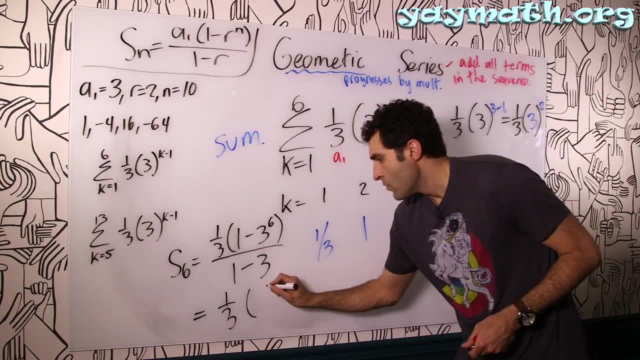 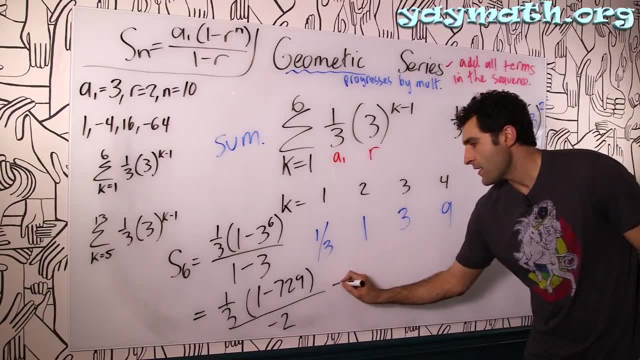 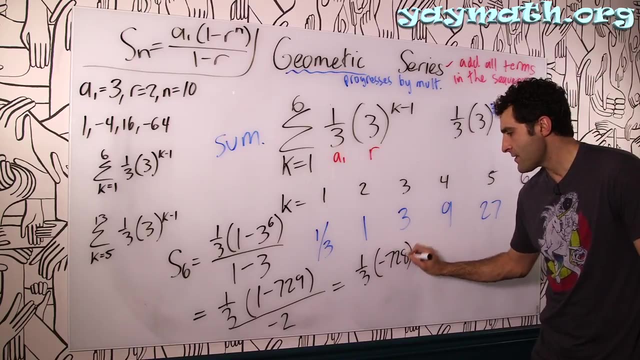 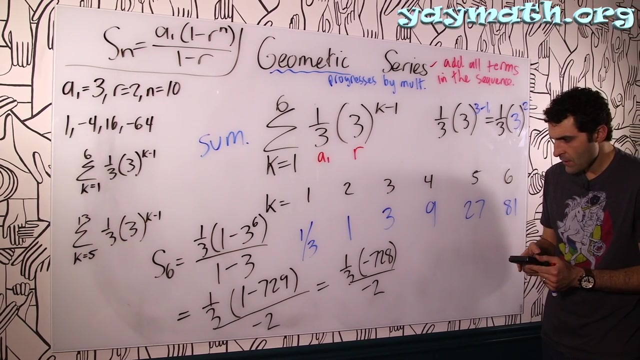 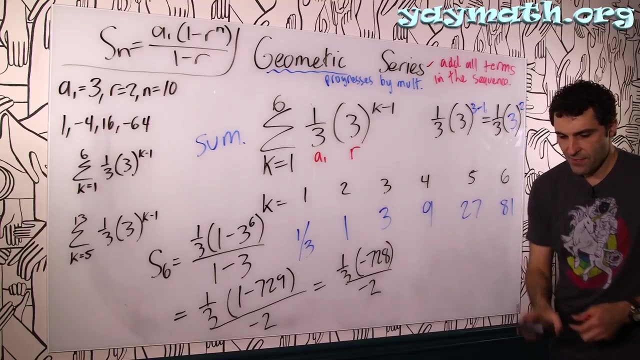 7 to 9.. 1 minus 7,, 29.. All over Negative: 2. This becomes 1 third times negative: 728 over negative: 2.. All right, I'm going to bust this out. on the calc, This is 7.. So you see, negative divided by negative will go away. 728 divided by 2. 364 times a third. 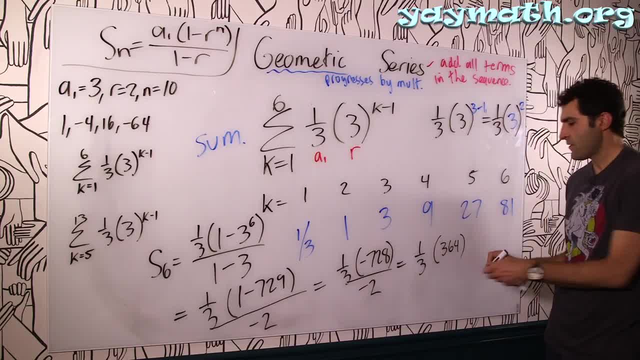 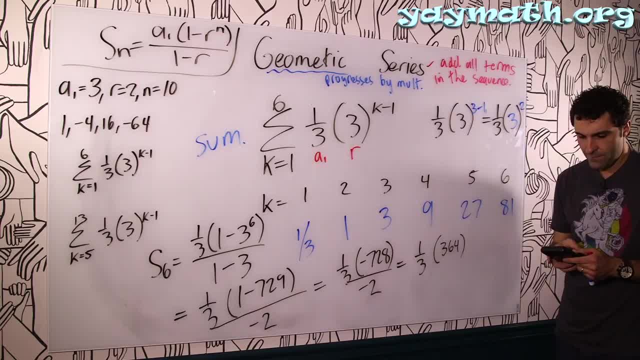 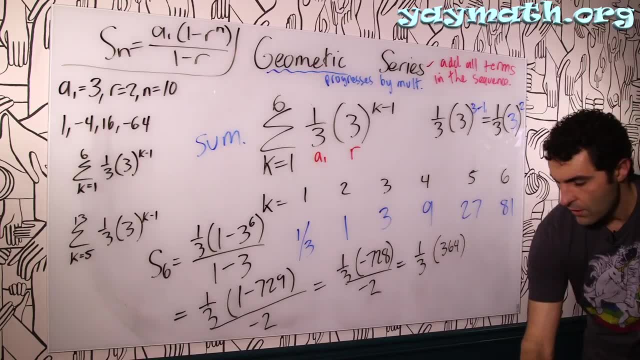 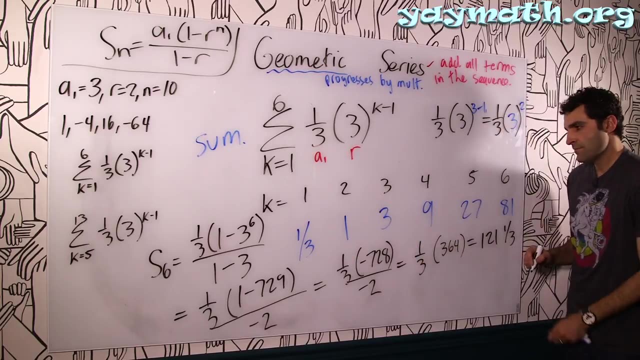 I don't think those. yeah, I don't think those do anything. All right, 364 divided by 3.. Yeah, it's 121 and a third. 121 and a third, Which I'm sure we would get if we add all these up. Yeah, we're totally going to get it Watch. 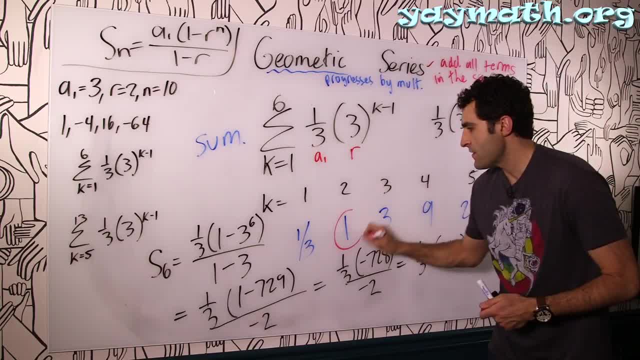 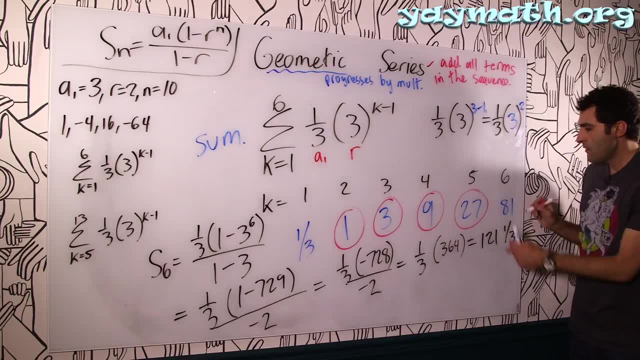 It'll be fun Again checking our answers. It's awesome. This is 10.. There's 10.. This is 30 more. That makes 40.. 40, 40 plus 81 is 121,, 121 and a third. it works. 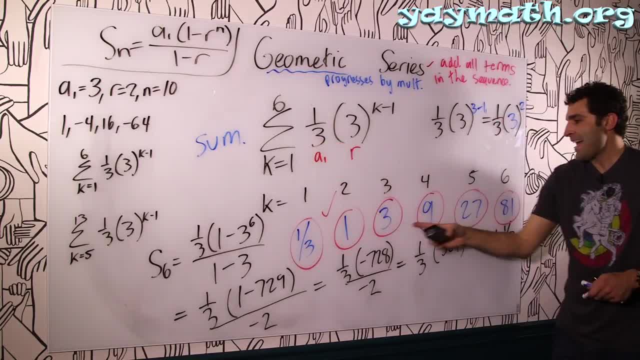 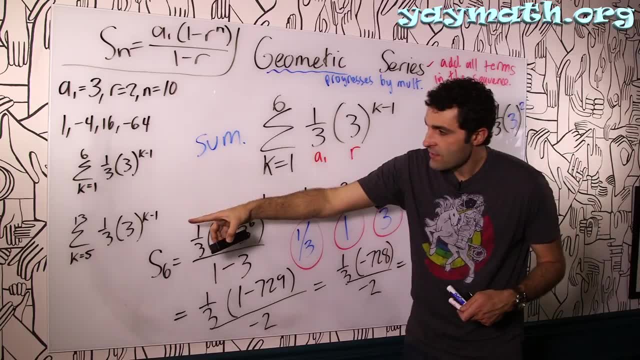 Okay, so now that's all sigma means. it just means add up these blue numbers in the sequence. We're gonna do this one here, and the good news is I did this on purpose. it's the same, but you'll notice the k is changing. 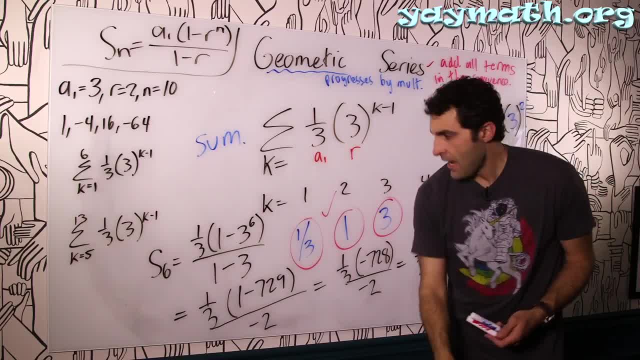 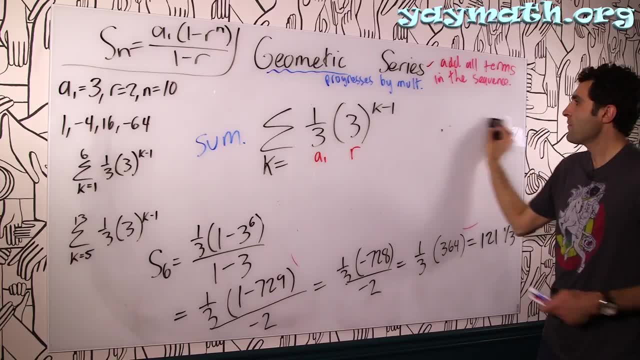 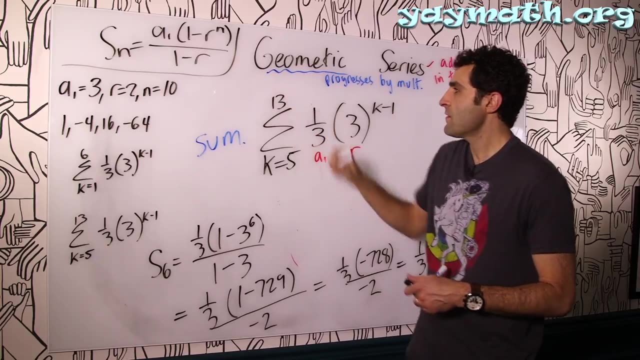 So I'm just gonna go ahead and take this off and this off here, and we'll even just take off the k work. There we go, We'll take that off, And now k ranges from five to 13.. So it's the same sequence we can assume. a1 is the same. 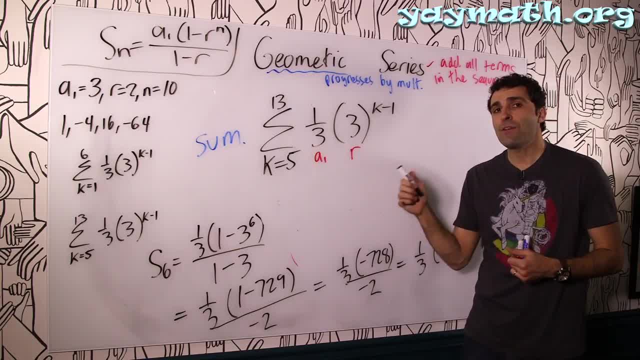 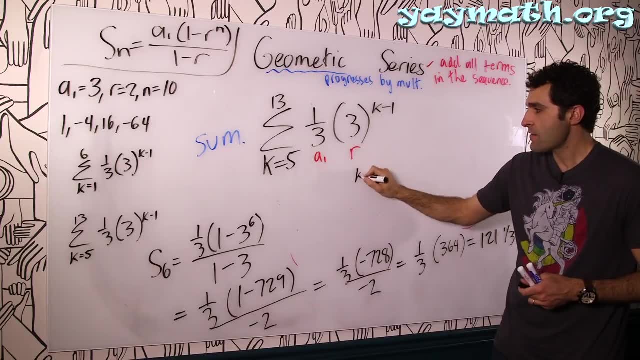 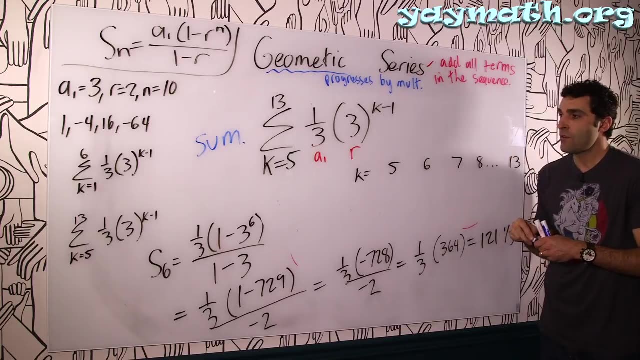 r is the same. however, this sequence progresses from when k is five up to 13.. So the definition of this sequence starts at five, then six, then seven, then eight, all the way from k equals 13.. So again, I would recommend getting a fix. 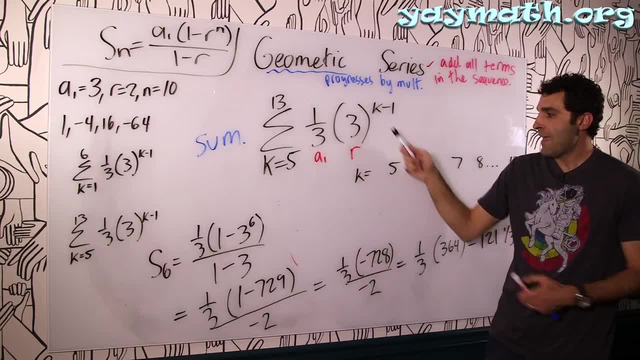 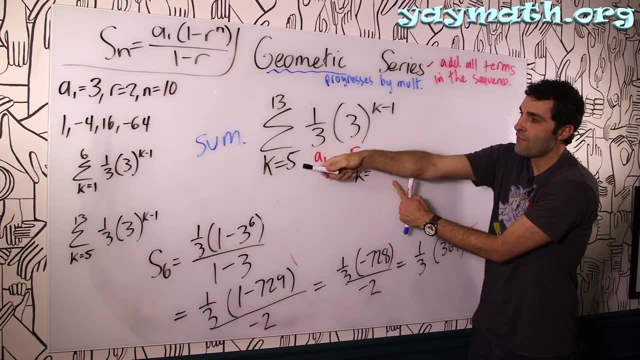 on what this sequence is. Let's put in five here, and that would be the first term in our sequence. all right, The first term in our sequence now is when k is five. The last term in our sequence is when k is 13,. okay. 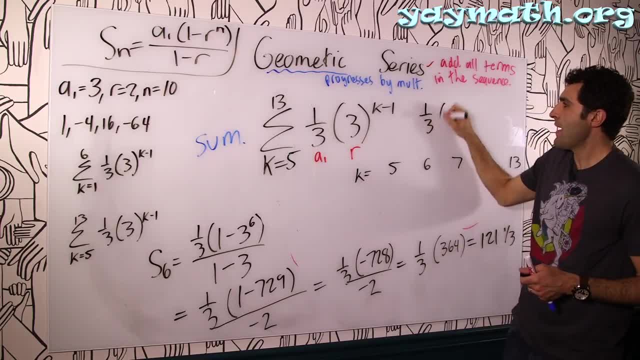 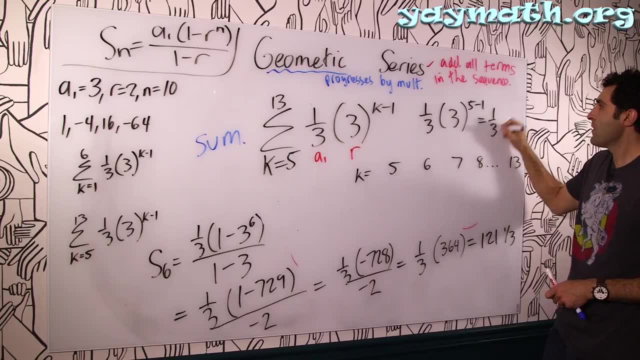 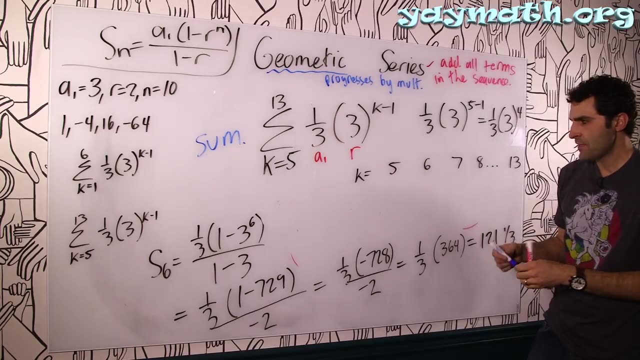 Let's go ahead and do that for one time. One third times three to the k, in this case is five minus one. This is one third times three to the fourth. I know three to the fourth is 81.. A third of that is 27.. 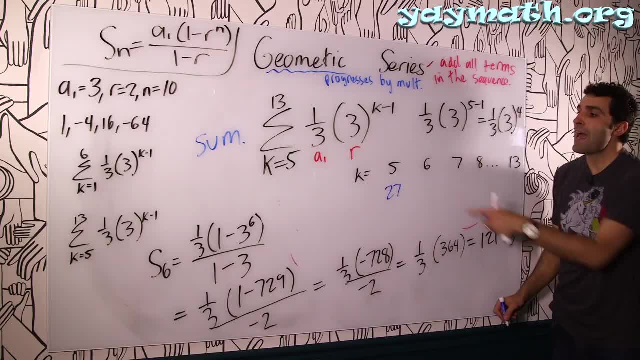 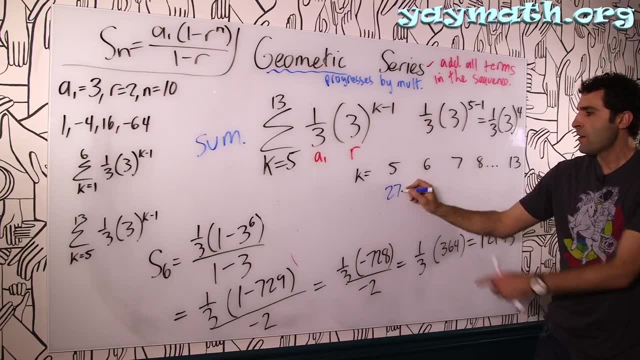 See what I'm doing: 27.. So now the first term in the sequence is 27.. The next term in the sequence is when k is six. right, Since r is three, we know, I'm just gonna multiply by three: 81.. 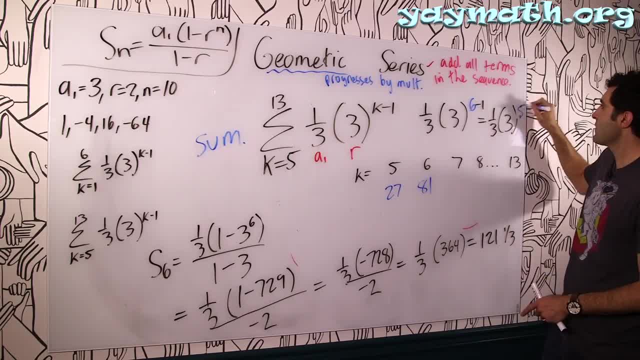 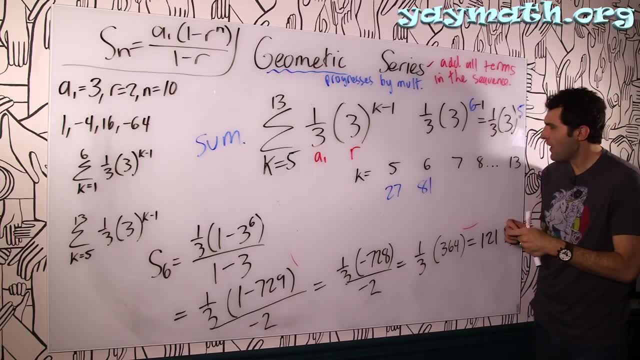 We'd get that here. k is six, there it is five. All right, So three to the fifth is 81 times three is 243, and a third of that is 81, right, All right, so that's fine. 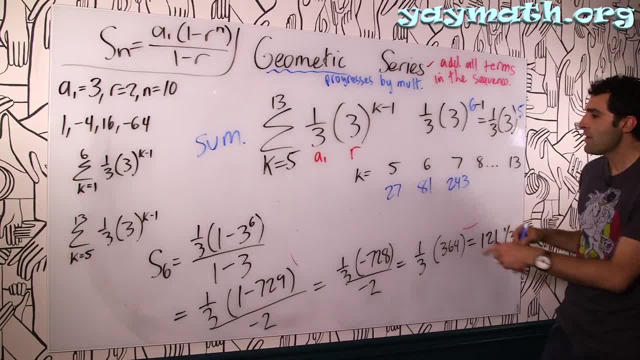 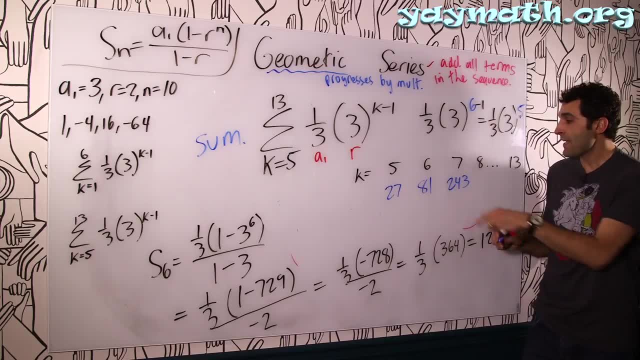 So we're progressing by three each time, just like before, except now the first term you would call is starting when k is five and the last term is when k is 13.. So we can get this sequence or the sum of it, the series. 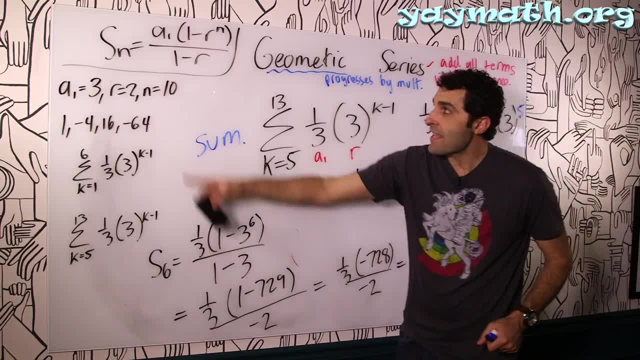 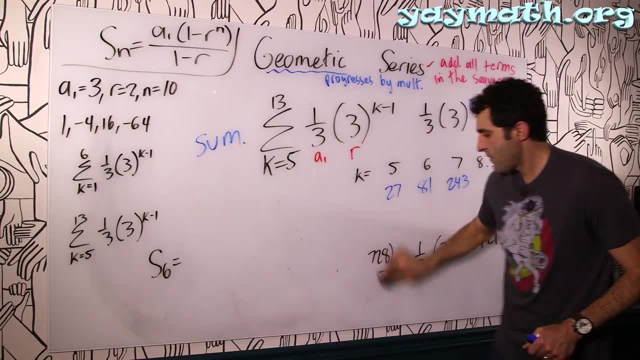 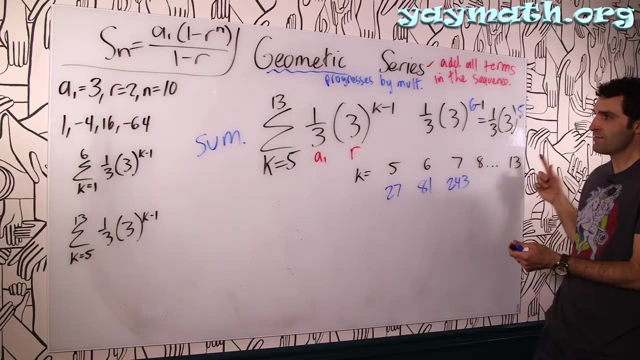 using formula again. So now look closely. Is a one still one third? No, Take this off, Take all this. now, Here it comes. Here's a question: How many terms are there Right? How many terms? So then we know what to ask. 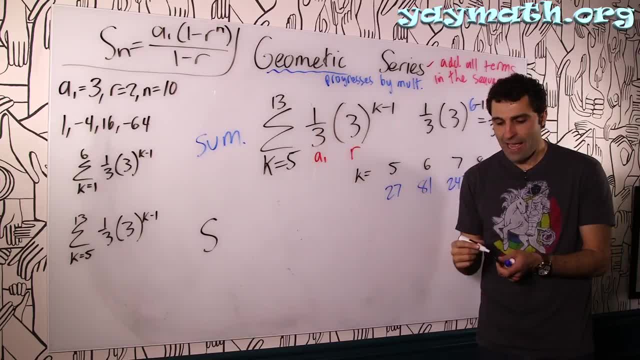 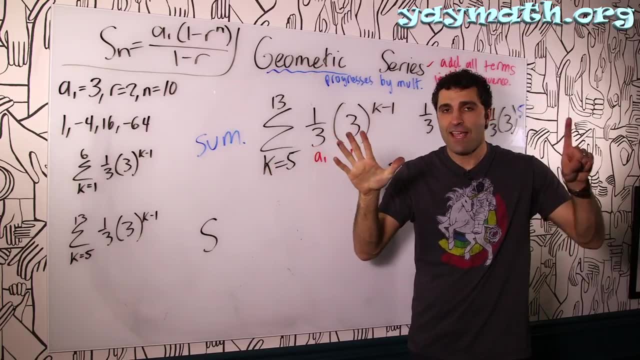 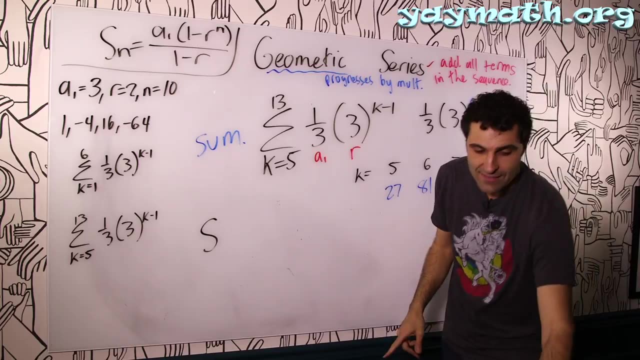 S what? Well, from five to 13 is how many. I'm gonna count them: Five, six, seven, eight, nine, 10,, 11,, 12, 13.. Nine terms in this sequence. Nine terms. 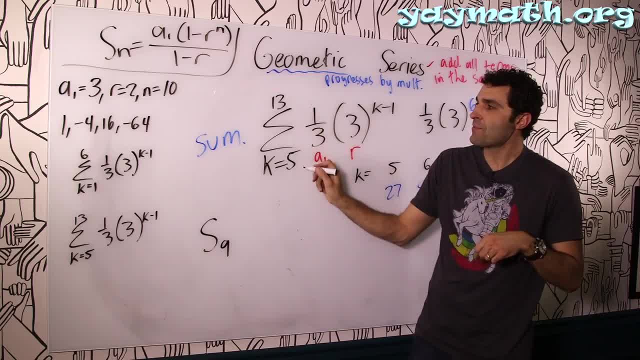 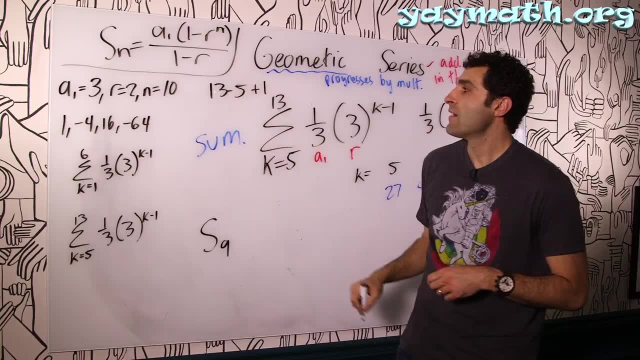 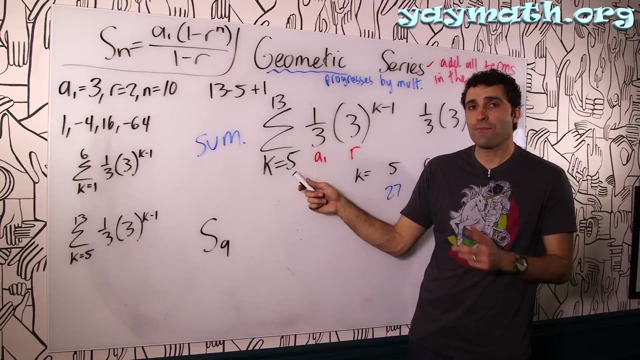 Does it make sense to you that it's basically the difference between these two, which is eight, but then added one to include both terms? all right, It's like, for example, if a teacher gave a homework assignment number five to 13,. 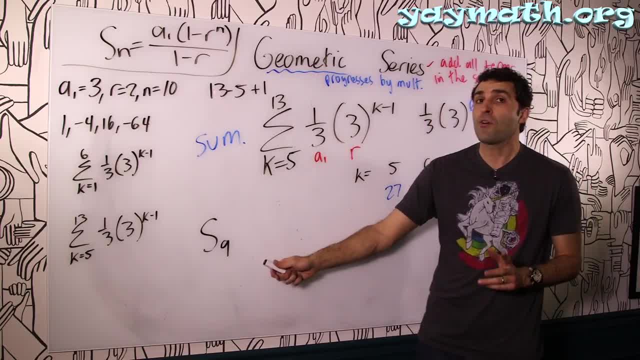 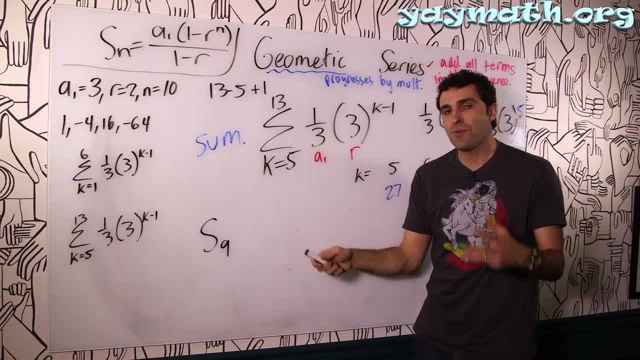 please do numbers five to 13.. You know that you're going to be gonna do eight. okay, You're gonna do nine to 13.. You've got to do nine to 13.. to be doing nine problems, right. Even though 13 minus 5 is 8, there's nine total numbers between. 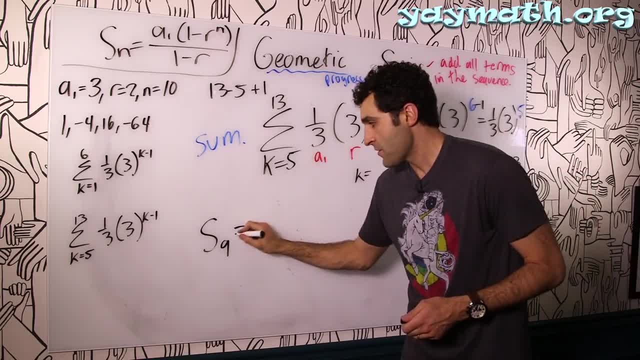 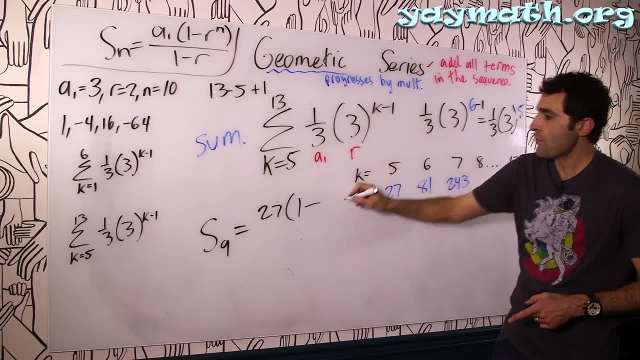 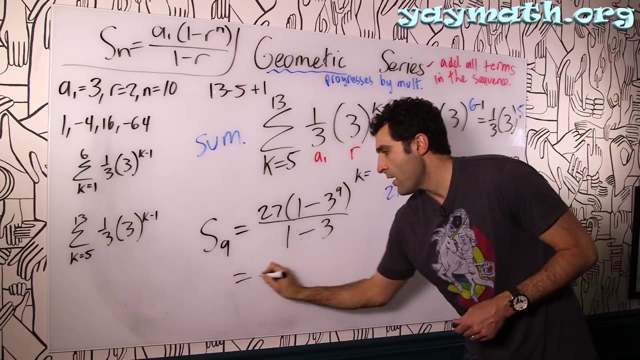 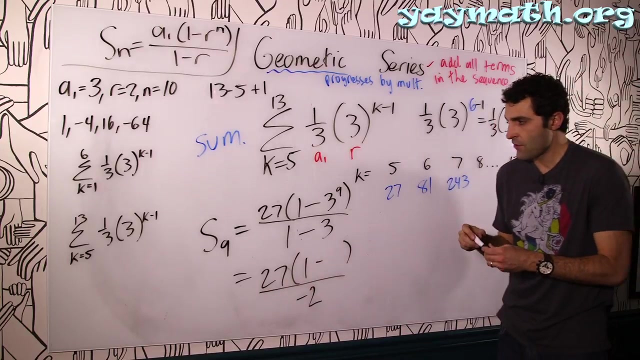 5 and 13.. It's kind of cool Equals, first term: 27. 1 minus rate: still 3.. How many 9 over 1 minus rate is still 3.. All right, 27.. 1 minus whatever. that is negative 2.. 1 minus 3 is negative 2.. 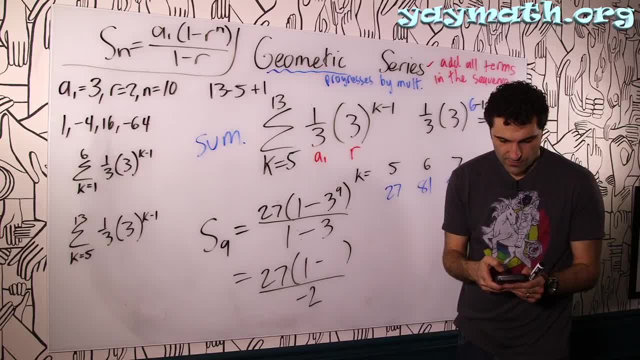 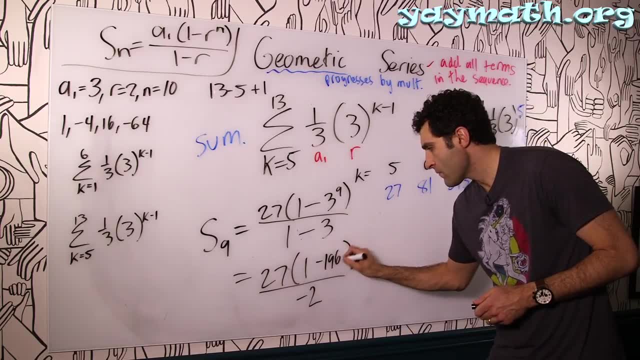 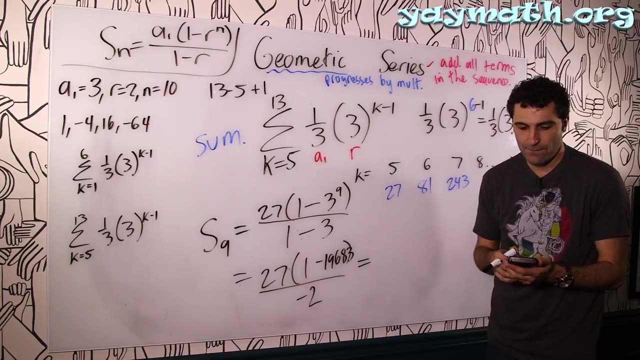 All right, let's get 3 to the 9 going. Here we go. Okay, 19,, 6,, 8,, 3.. There it is, And you know what? I'm just going to use calculator time. Here we go. We got 1 minus. 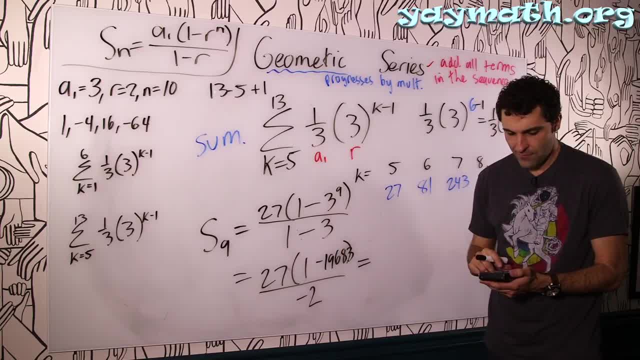 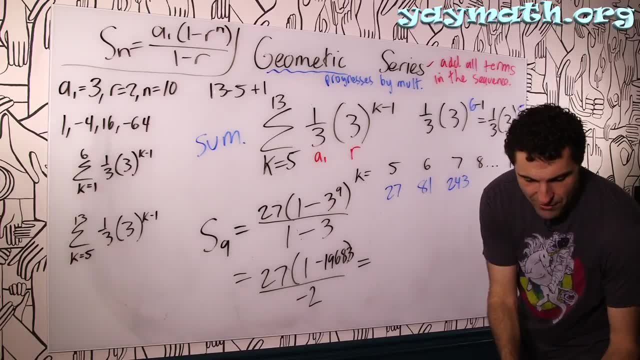 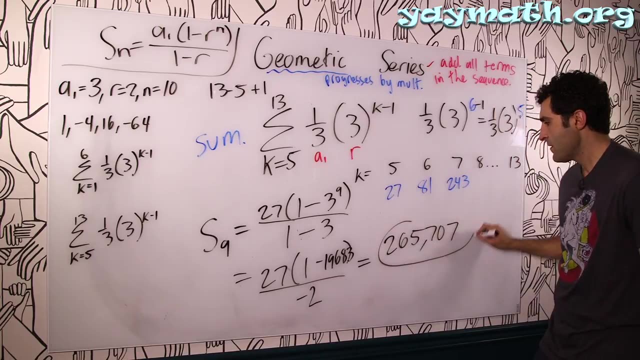 that. There it is, Times 27.. There it is Divided by negative 2. 265, 707.. It's kind of amazing, huh, Wow, look at that. You know, if you start at 27 and go up to 9 terms,